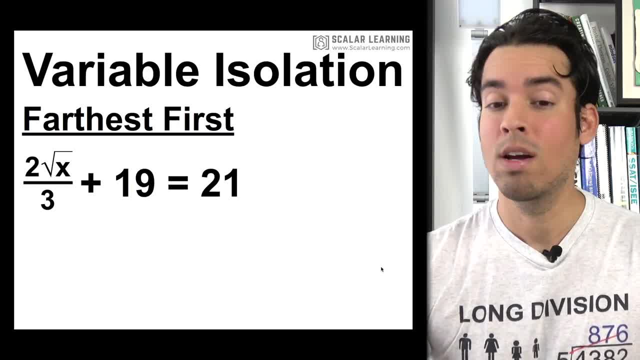 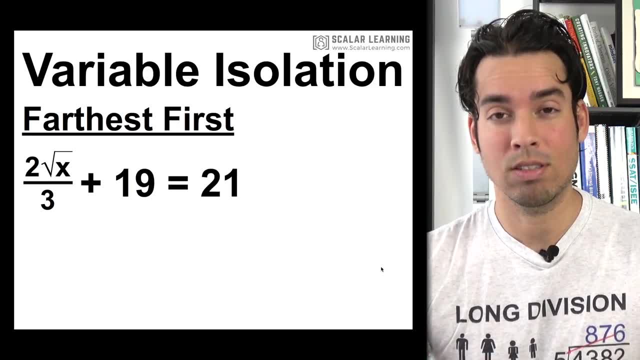 square root of x divided by three Plus 19 equals 21.. I want to get that 19. I want to get that 3, the 2 and the square root all out of there, so the x can be by itself as its own entity. 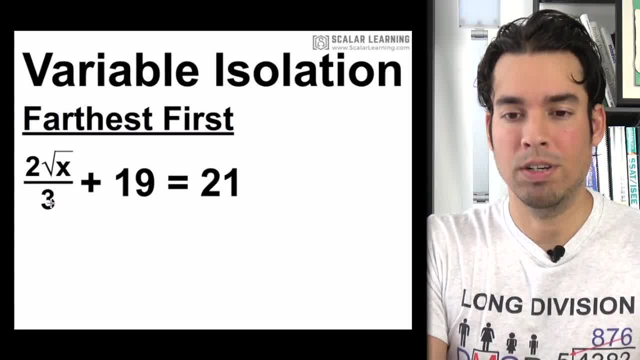 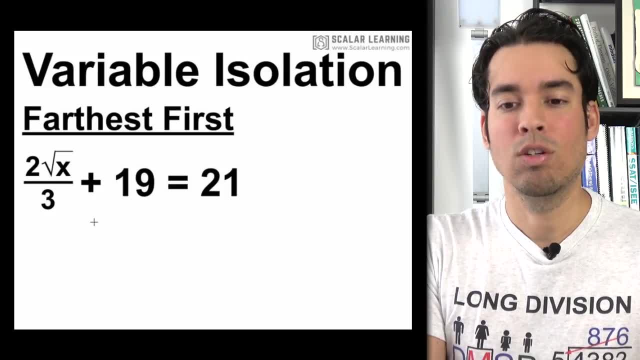 So this is how we're going to run through and kind of attack this problem here. So first, what I'm going to do is I'm going to see what's farthest from the x first. Not that 2, not that square root, not that 3, it's the 19.. So we're going to start by doing the inverse of adding 19, which is subtracting 19.. 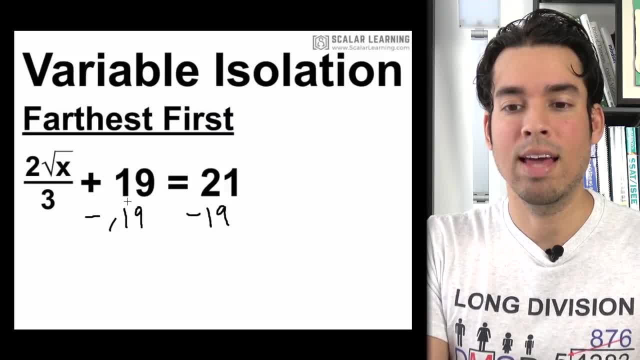 I'm going to do it from both sides. we're going to subtract 19 from both sides. That cancels out and, of course, now I'm left with 2 radical x over 3 equals 2.. Excellent, Now what's the next thing? Well, the 3 is the next thing. that is farthest away, right? 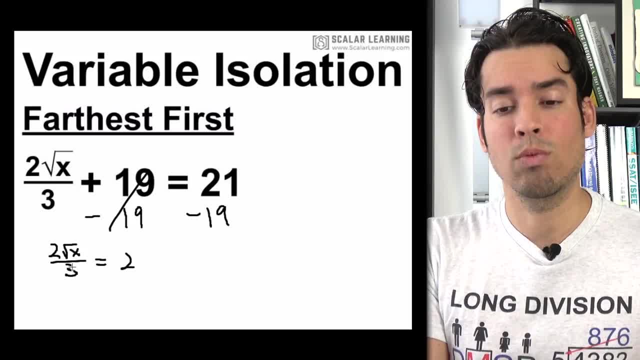 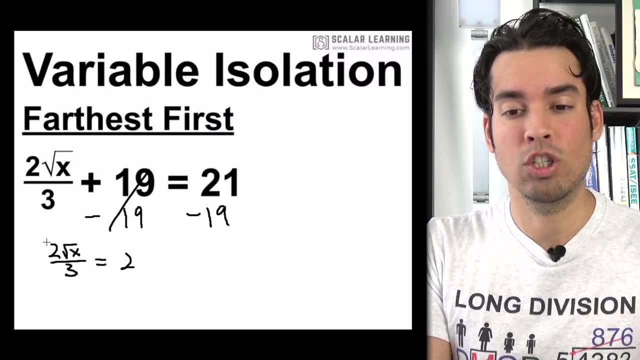 The 2 is on the same level, the square is happening right directly to the x. So I want to get rid of that 3.. Currently the x is dividing that 3, dividing by that 3. So we want to do the opposite of division, which is multiplication. 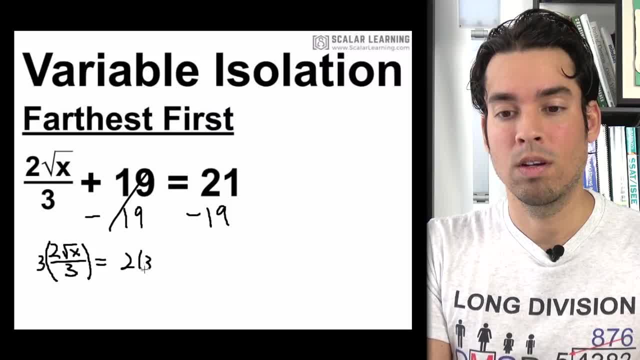 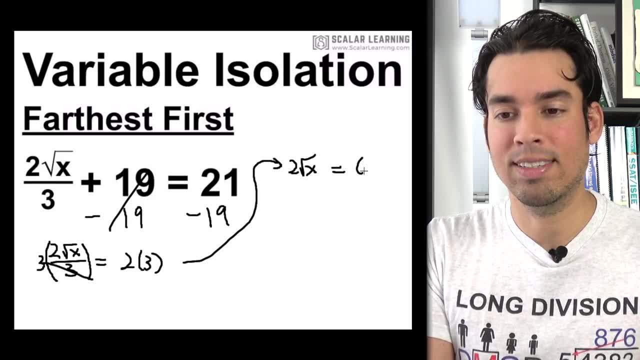 So now we're going to multiply both sides by 3. And in this case These cancel out and we get 2. radical x equals 2 times 3, which is 6.. Now I want to get rid of that 2 right. 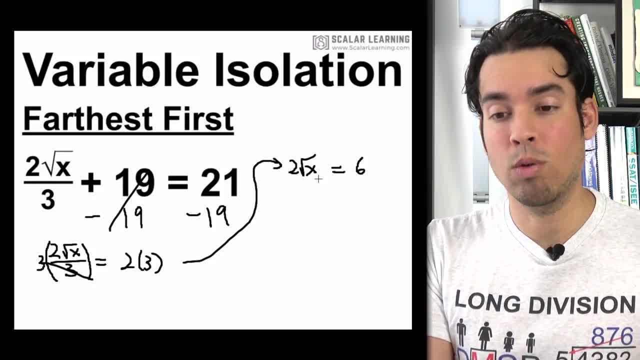 The square root is going to be the last thing we're going to get rid of. I want to get rid of the 2.. The 2 is multiplying this quantity, So we're going to divide by 2.. That's the inverse operation of multiplication. 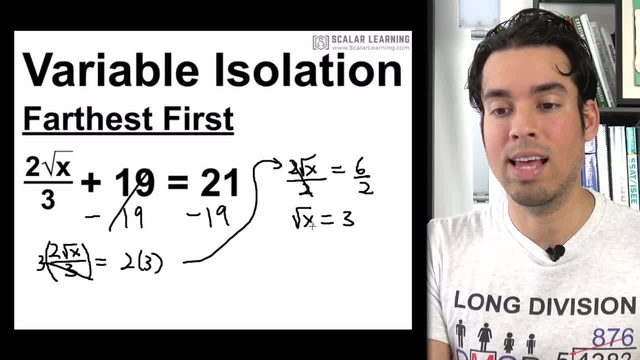 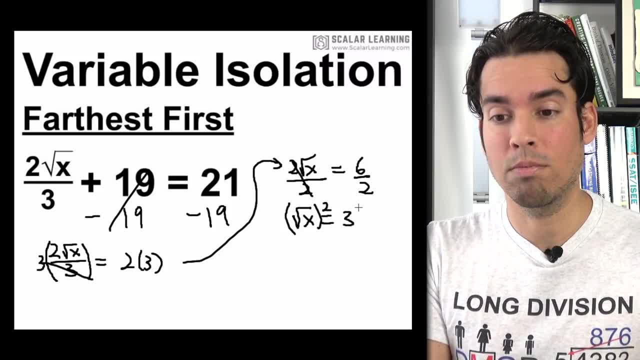 And I get: square root of x equals 6 over 2, which is 3.. And, last but not least, we need to undo the square root. I need to get rid of that square root. What's the opposite of a square root is squaring both sides. 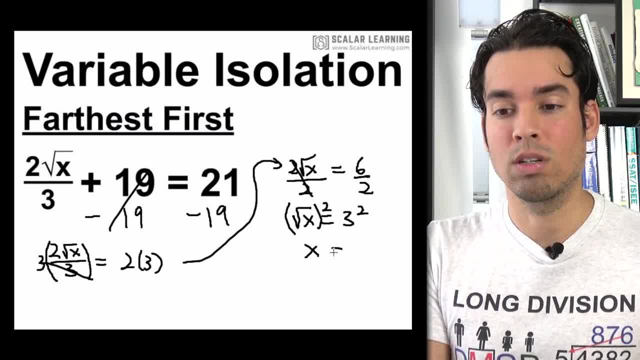 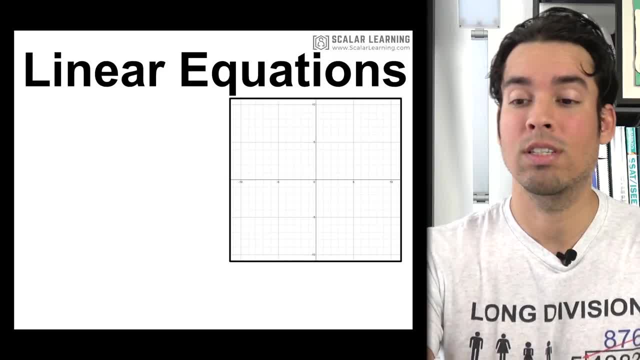 Square root of x squared is just x, and then 3 squared is, of course, 9.. And there's your answer. Next, we're going to talk about linear equations, And a linear equation is simply an equation of a line. So here are a couple examples on this graph of linear equations in terms of their formulas. 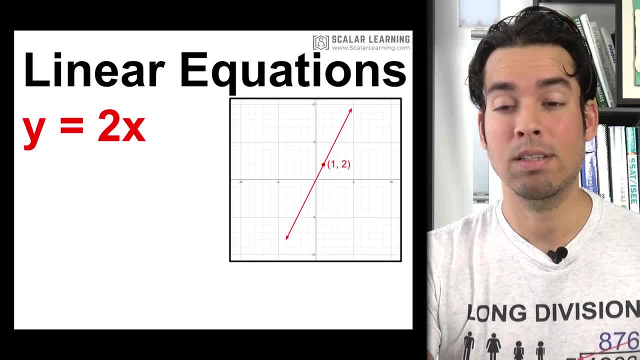 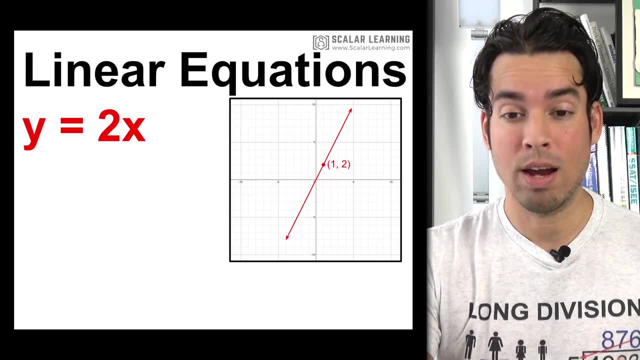 and what they look like. So here's: y equals 2x, A very basic linear equation, And you can see that point 1 comma 2 falls on the line And that makes sense. If I plug in 1 for x, I'll get 2 for y. 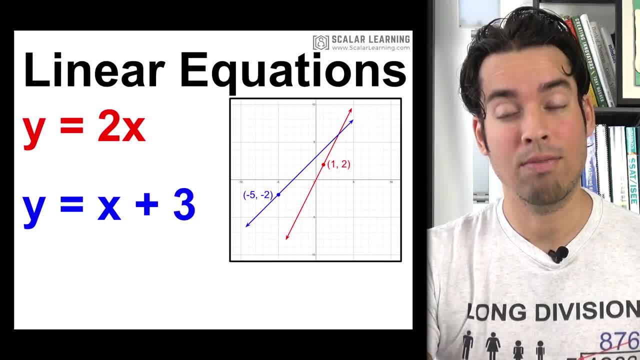 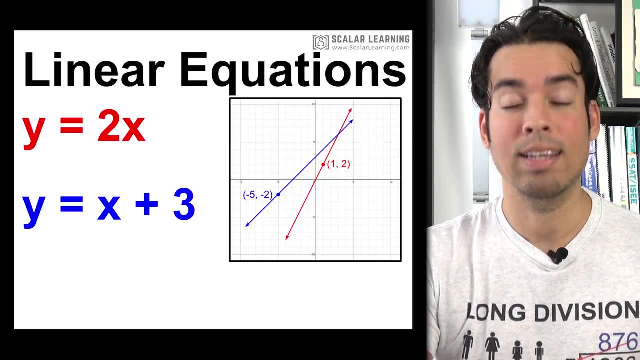 Next we have y equals x plus 3.. And notice again, I've called out that point: negative 5, negative 2.. So again, if I take that negative 5 x value, plug it in for x, I get negative 5 plus 3. 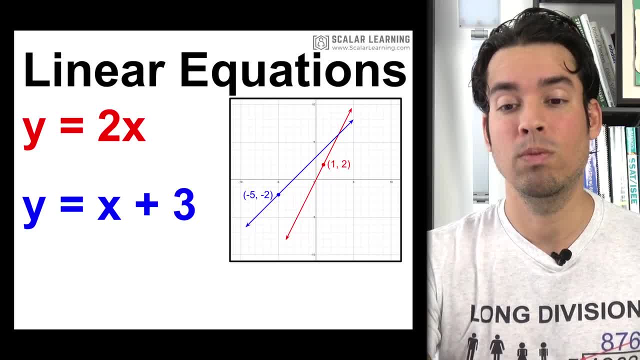 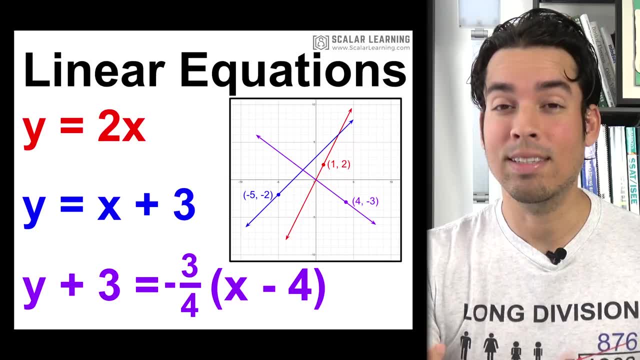 which equals the y value of that coordinate negative 2.. And last but not least, a little bit more complex one We've got: y plus 3 equals negative 3, fourths times x minus 4.. That, again, is simply just a line. 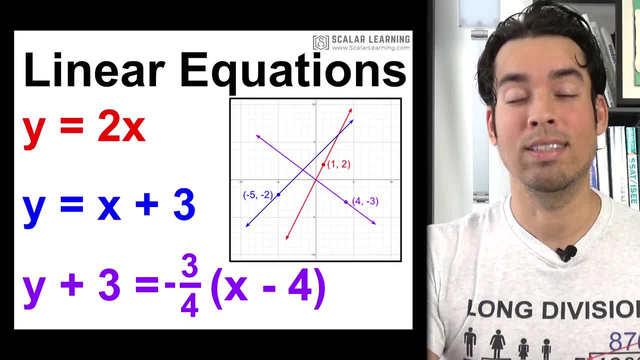 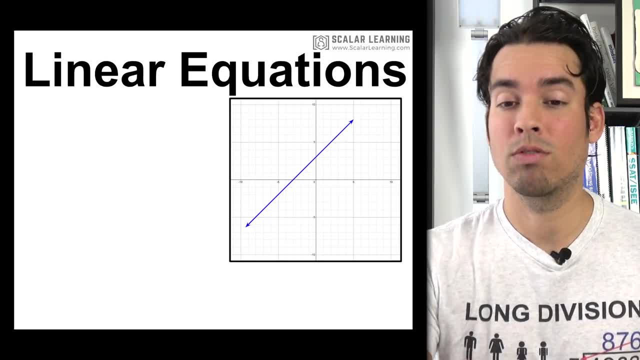 And this one has a negative slope, So you kind of see it going down from left to right. Now, when we talk about linear equations, there are a few points and values that we have to be aware of. So these are the critical values, and these are especially important when it comes to 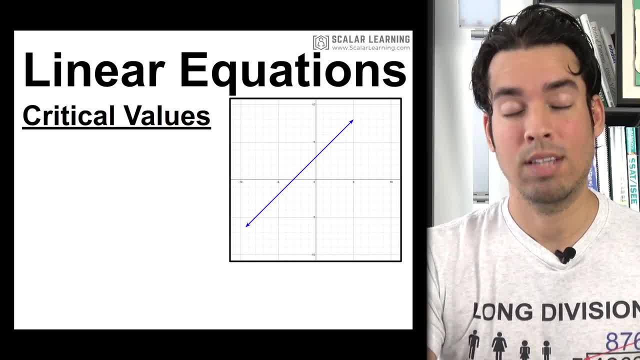 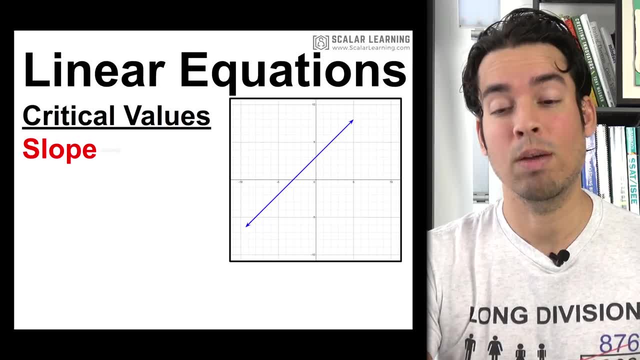 word problems or interpreting linear functions. So we again- I've taken one of the lines from the last example And I want to identify these points. So the first thing we have to identify is slope. And what is slope? Slope is rise over, run between any two points on the line. 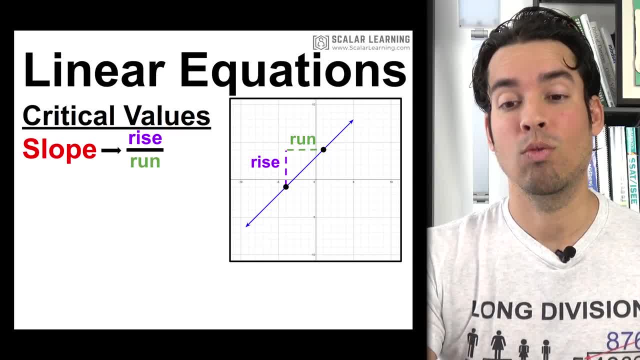 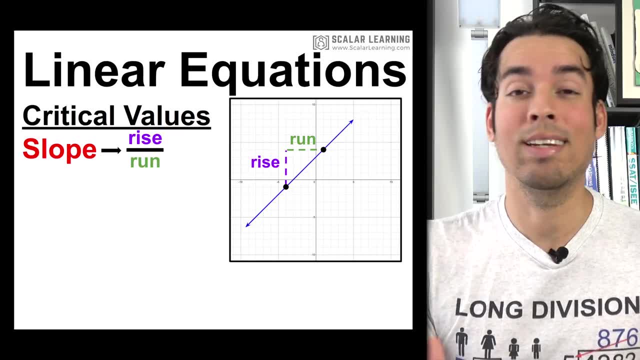 So here I've chosen two points that are easily identifiable, And to get the slope I'd simply take the rise, meaning the distance I'm going up over the run, which is the distance I'm going across to get from one point to the next. 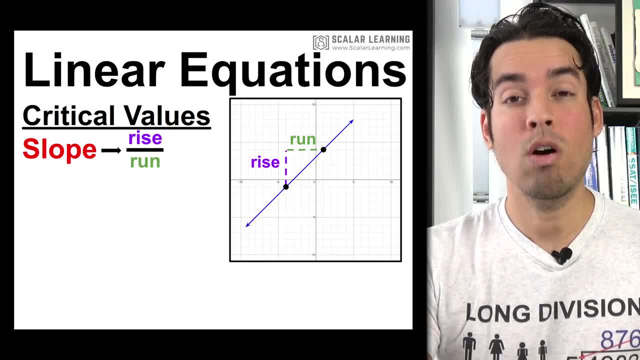 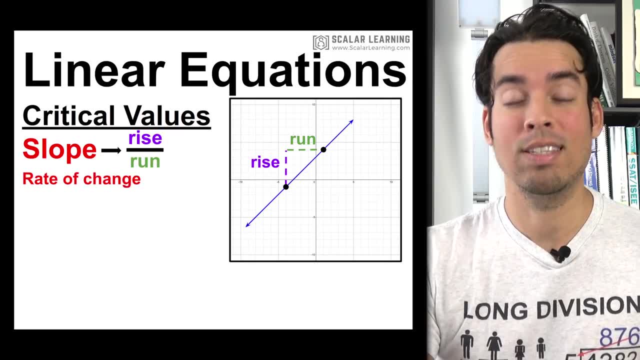 And I'll go into more detail on that in the next slide. When we're talking about a word problem, where we're trying to interpret a linear function, the slope value is always the rate of change. It's the amount that the y value or the final value is going to change every time the x 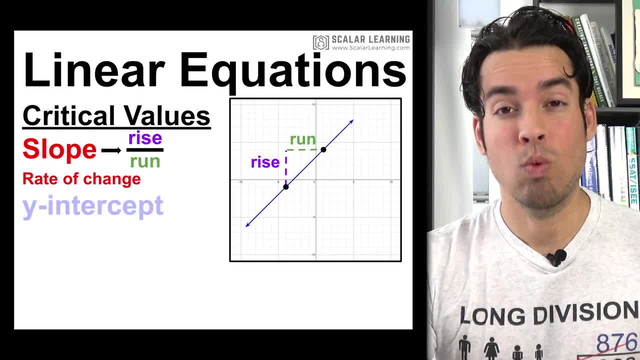 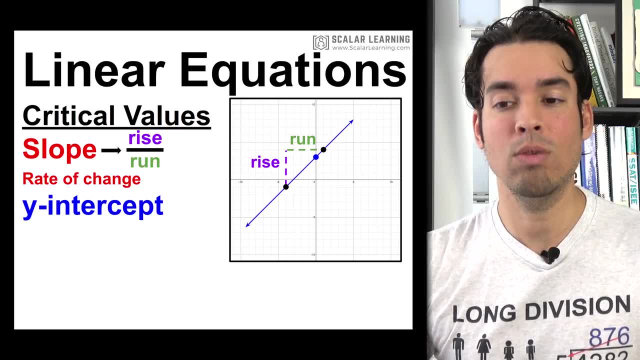 value usually increments by one. Now let's talk about the y intercept. The y intercept- The y intercept, as you can see on the graph right here, is where it hits the y axis. So this is literally where it's hitting the y axis. 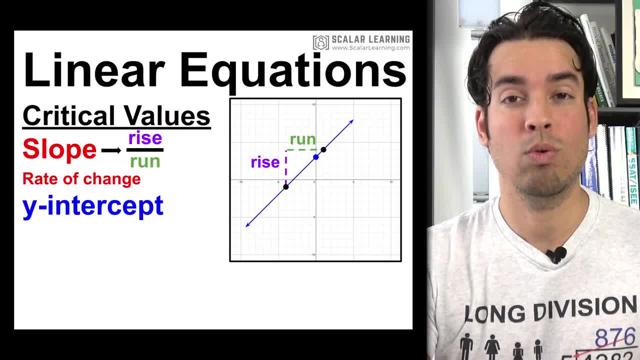 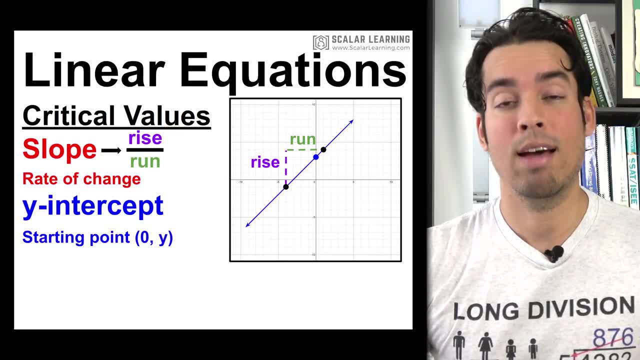 And the way we think about this. when we're interpreting a linear function or a linear equation, it is usually our starting point. It's our starting value, our initial value. If we think about a gym membership, where we have a fee that you pay to sign up and then 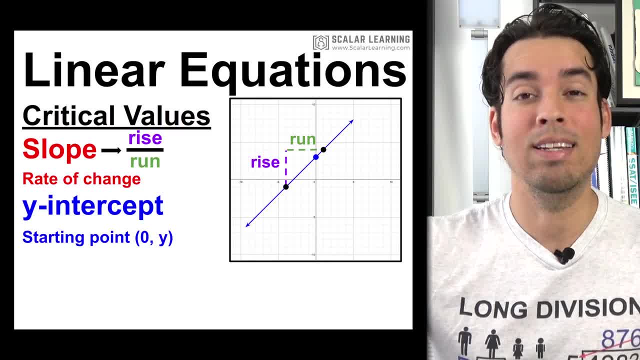 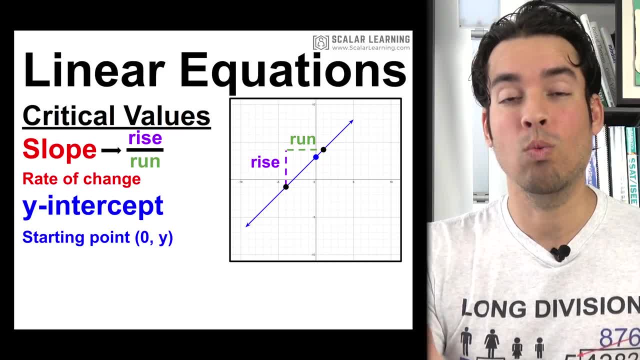 a monthly fee. the monthly fee would likely be the slope And the initial payment. the one time fee is going to be the y intercept And again you can see that The x value of the y intercept is always zero. Finally, we come to the x intercept. 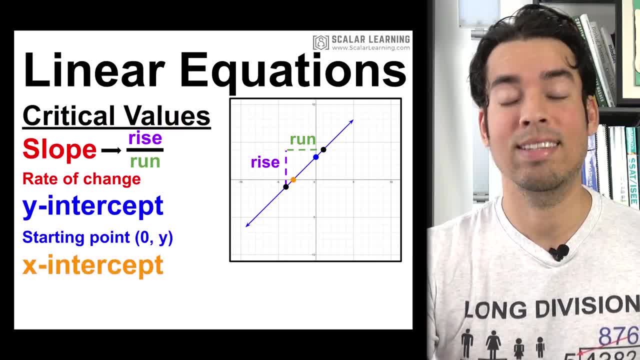 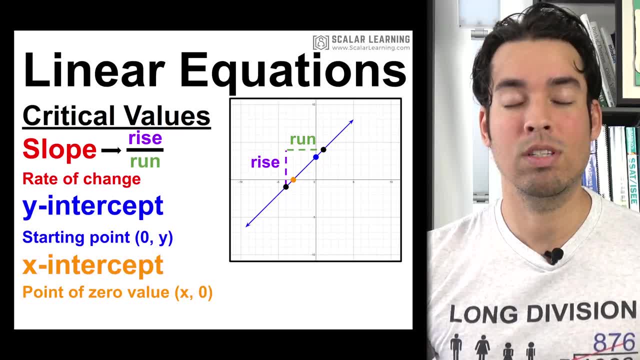 So the x intercept, as you can see on the graph, is where this function intersects the x axis, And usually how we interpret this in a linear function or linear equation is: it's the point of zero value. It's where we're hitting zero. 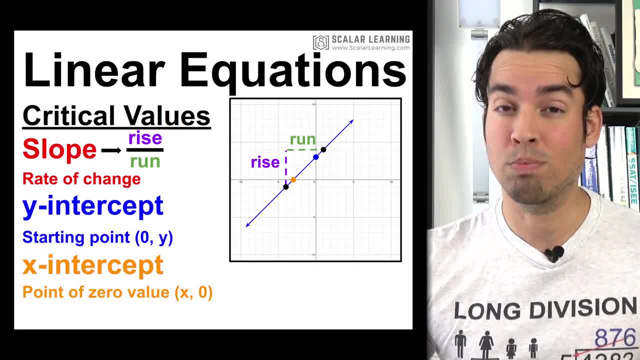 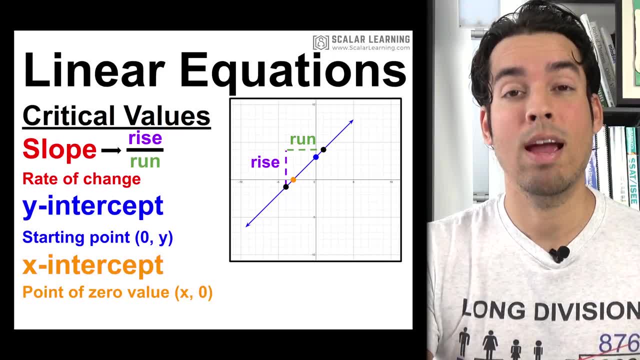 So, for example, if we're talking about a linear function that represents profit, the x intercept is going to be the point at which we have a zero profit. Lastly, we can see that for every x intercept, The y value will always equal zero. 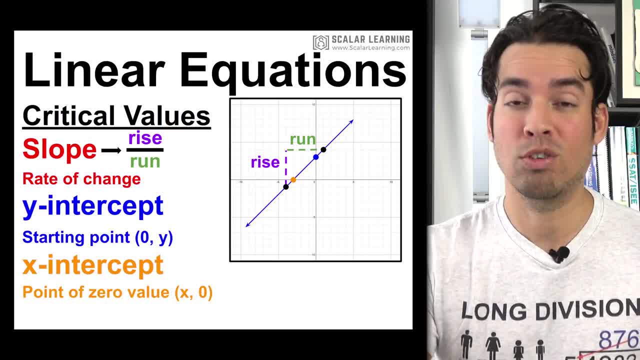 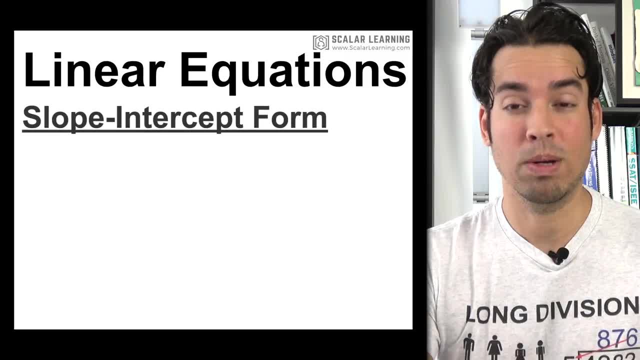 So if we have an equation, we're trying to find the x intercept, Just plug zero in for y. Now we're going to talk about the different forms for linear functions, And first and foremost is slope intercept form. This one you've got to know. 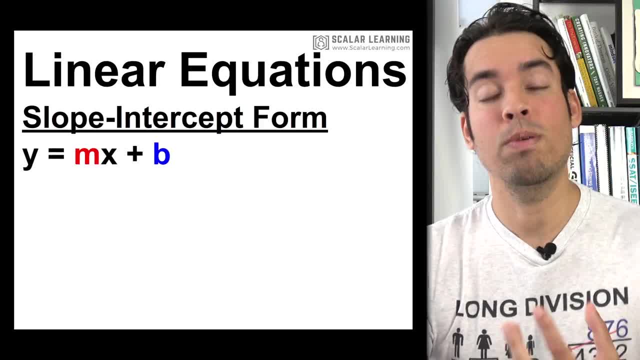 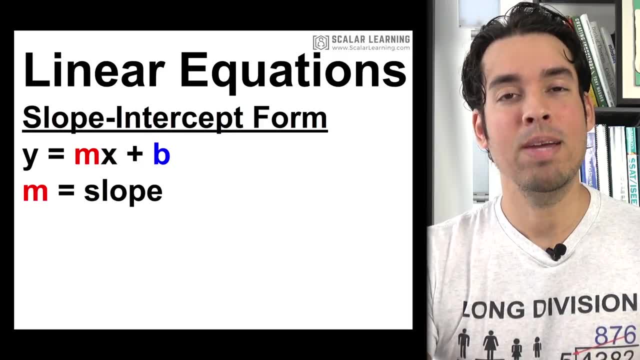 It's tested extremely frequently on the SAT. So slope intercept form is: y equals mx plus b. Make sure to burn that into your brain. And in this case the m is slope and the b is your y intercept. So it means that When y is isolated, 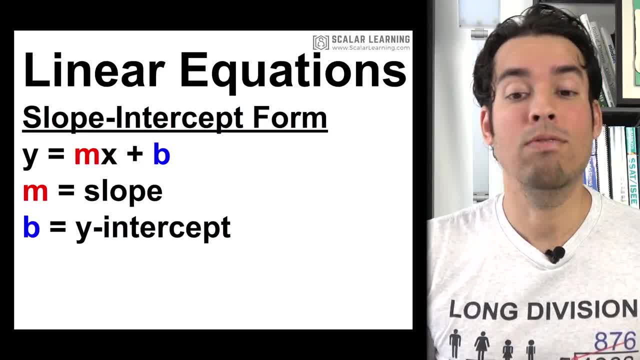 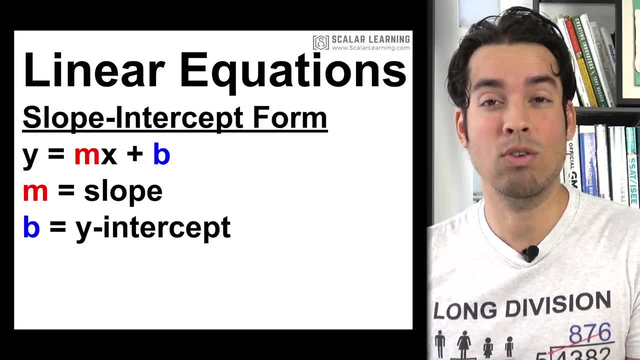 And we've got a linear function, a linear equation. Whatever number is next to the x value is going to be our slope value, which again was rise over run, And whatever constant is out there by itself is going to be the y intercept. 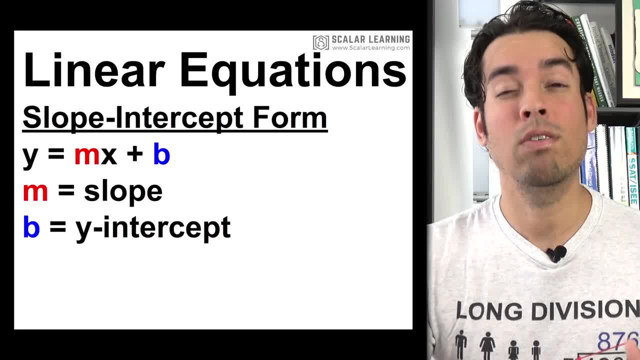 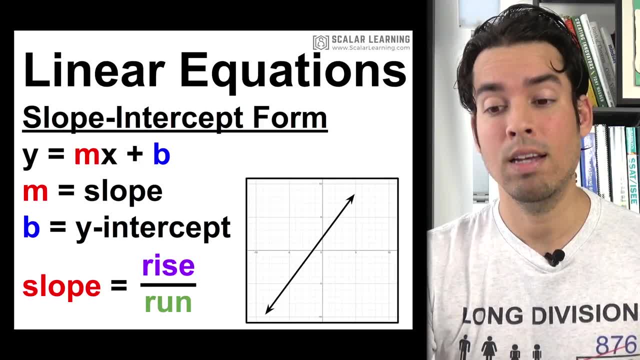 Again where this function crosses the y axis. So to just get a better visual understanding of what the slope means when I'm saying rise over run, let's take another example where we have a graph, we have a line, And again I'm choosing two arbitrary points. 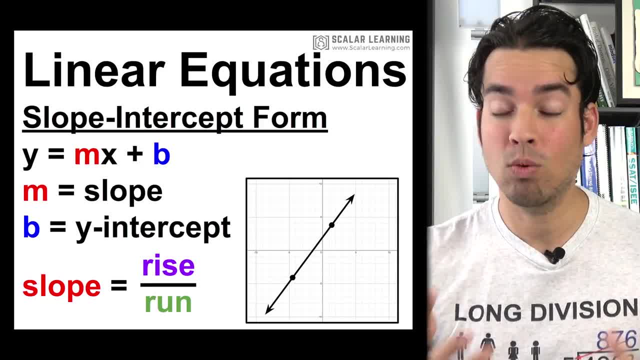 That's the beauty of it: The slope will always stay the same. for a linear equation, It's going to be a linear function. It doesn't matter what these two points are. but I'm choosing two arbitrary points And I'm just looking at: hey, that's the rise. 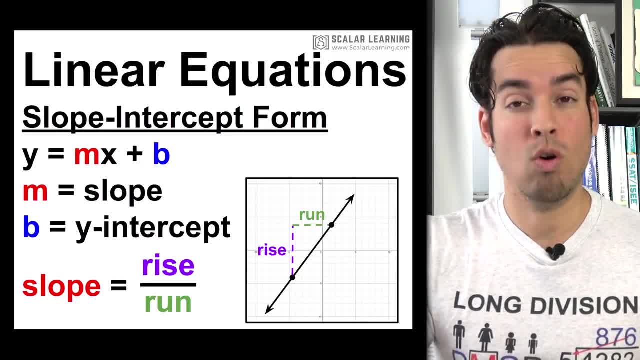 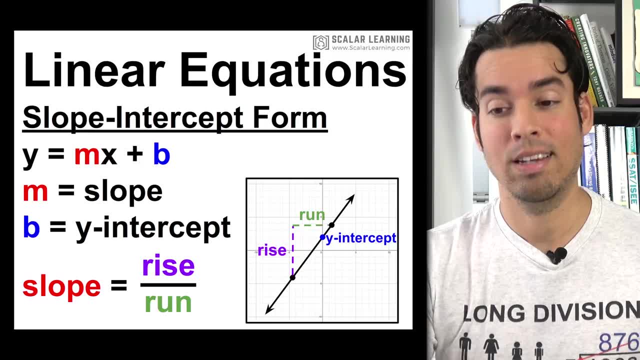 That's the run. The slope is the fraction of the rise over the run value. And again, just to get more familiar with what the y intercept is, it's that point right there where we're intersecting the y axis. So now here's an example of slope intercept form in action. 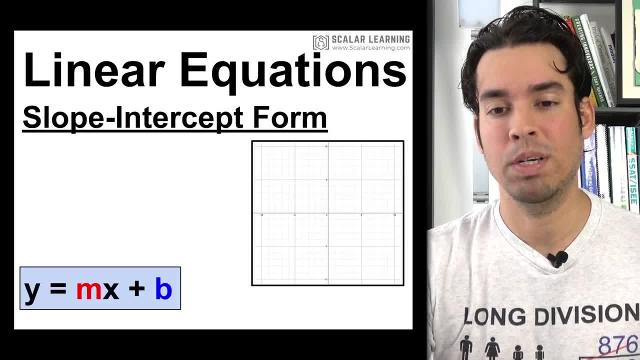 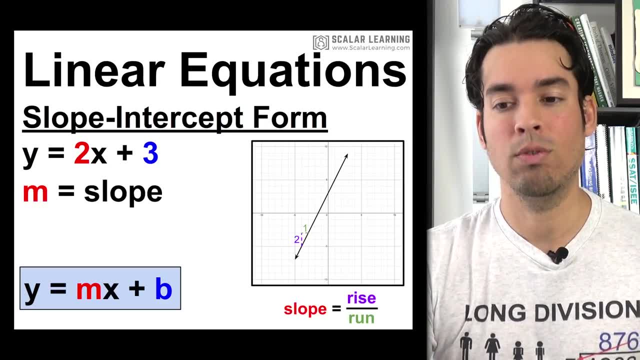 Again, I've got the baseline equation: y equals mx plus b. So let's say we have the graph of y equals 2x plus 3.. So you'll notice The slope is that 2 value And we can see the rise over run of those two points. 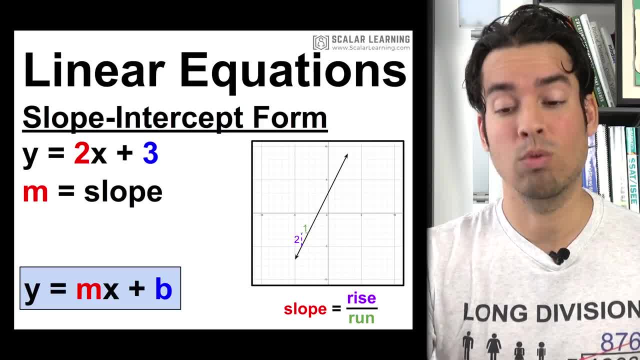 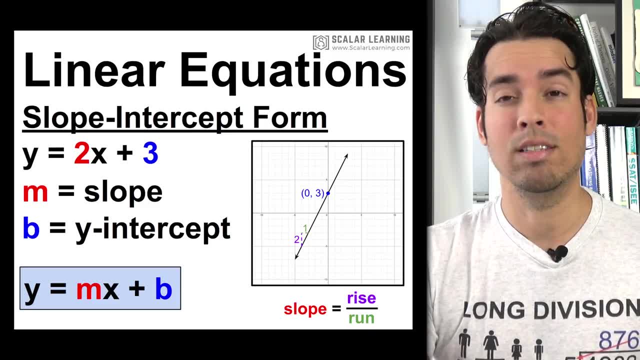 It's 2 over 1, which 2 over 1, of course equals 2.. And that b value, that blue value, is the y intercept, And you can see it crosses the y axis at 0 comma 3.. 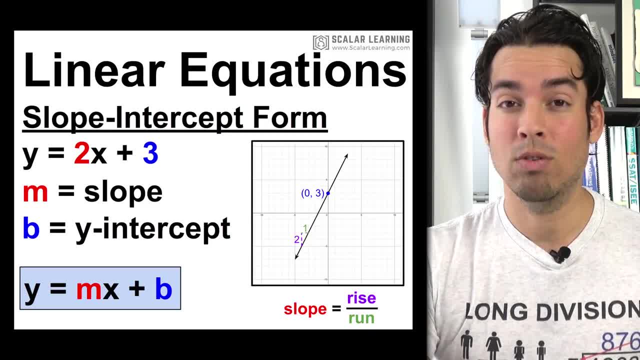 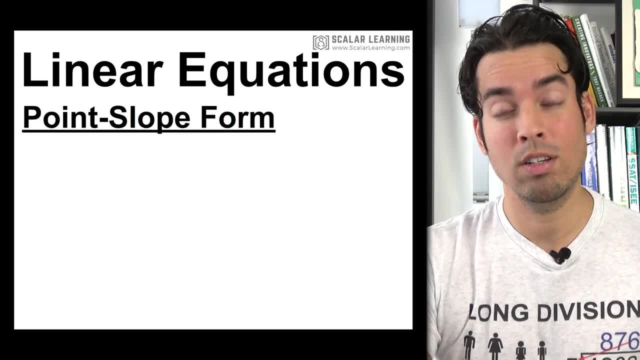 And you remember I said, every time you have a y intercept, the x value is going to be 0. And that, of course, is holding true here. Next, we're going to talk about point slope form, So this is another one that you've got to know. 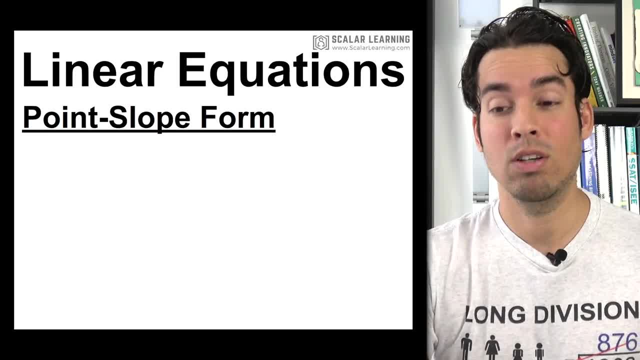 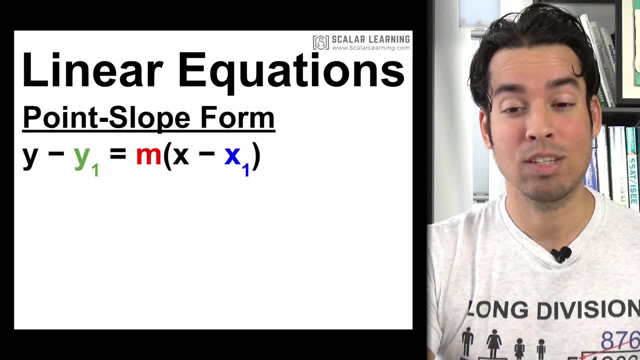 It's not as important as slope intercept form, But I would say to definitely know this form. So in this case the format for the equation is: y minus y1 equals m times x minus x1.. And once again the m value is slope. 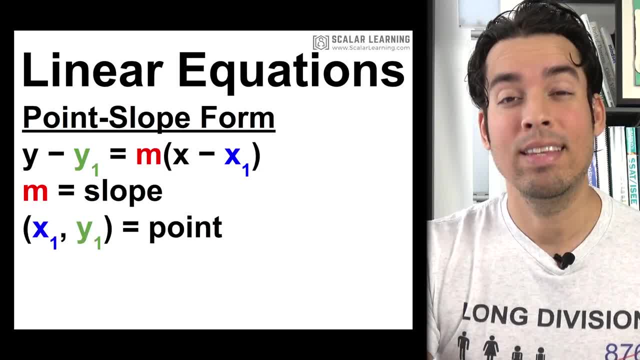 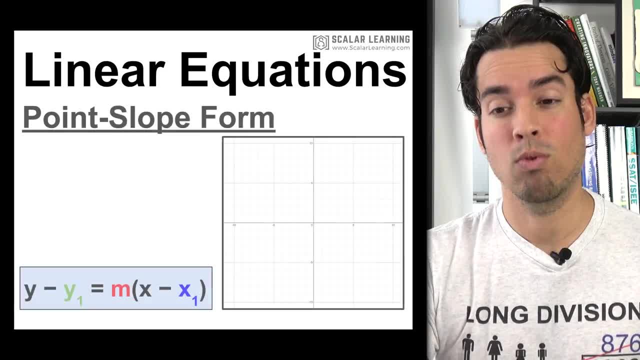 And the x1, y1 values are simply the coordinates of any point of this line. You can choose anything and it'll still be a valid equation. Now here's an example of point slope form, And again we've got the graph up there and we've got the equation at the bottom. 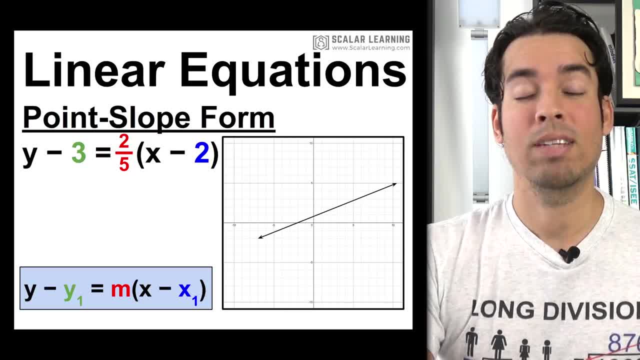 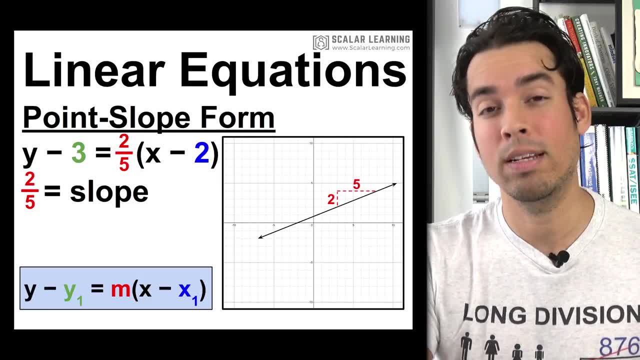 So I've got y minus 3 equals 2 fifths times x minus 2.. So in this case, again, that 2 fifths represents the slope. It's going up 2 and to the right 5, right, That's always going to be the ratio up 2 to the right 5.. 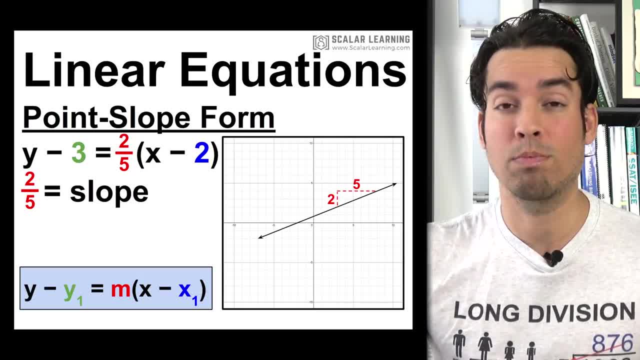 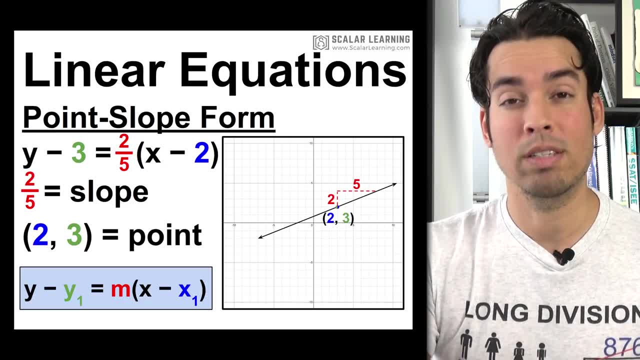 Even if it went up 1, it would go to the right by 2.5.. So it's a proportional relationship. And then there, of course, is that coordinate that we see up there. That 2 value and that 3 value represent a 2 comma 3 coordinate. 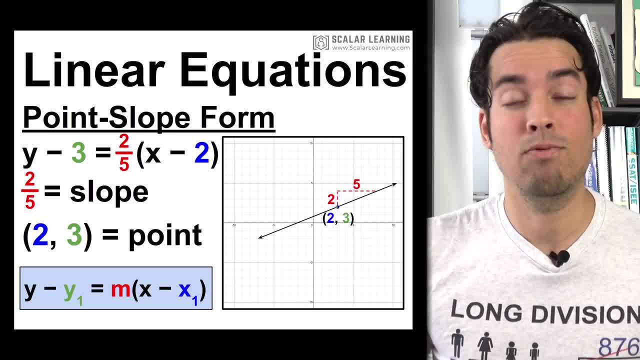 And you notice that's a positive 2 and a positive 3.. But in the format of the equation we're always subtracting those values, So we're going to do that. So if it was a negative value it would actually turn into a plus. 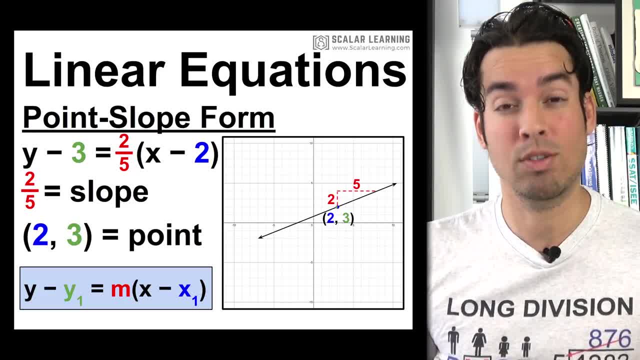 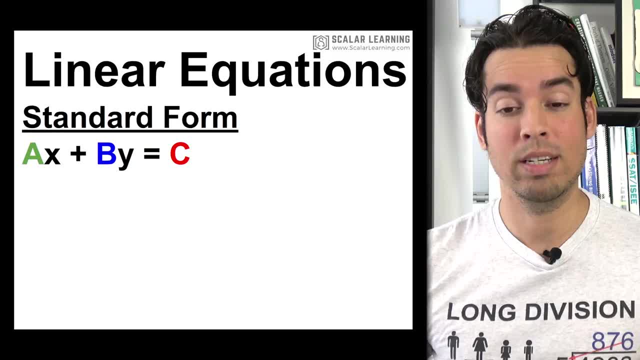 If it were a negative 3 there for the y value, it would be y plus 3.. Next we're going to come to standard form. So what is standard form? Standard form is when a linear equation is written in this format: ax plus by equals. 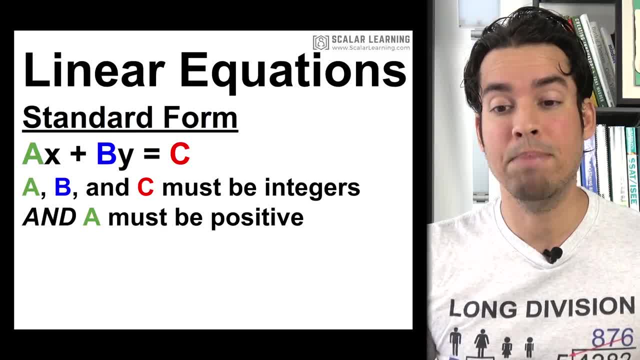 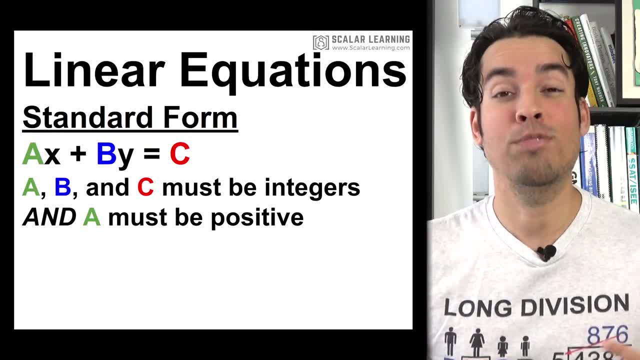 c. To be a valid standard form, a, b and c must be integers and a must be positive. This doesn't mean that b and c have to be positive. This just means that a must be positive for it to be the value. 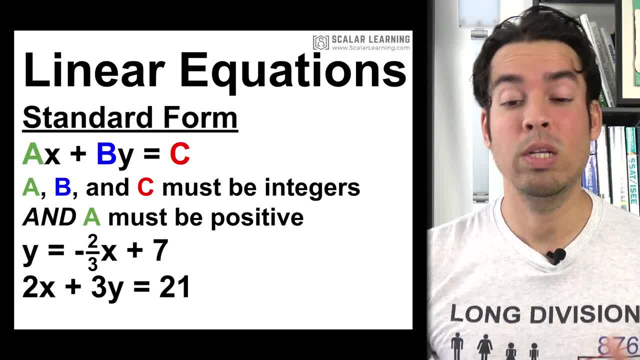 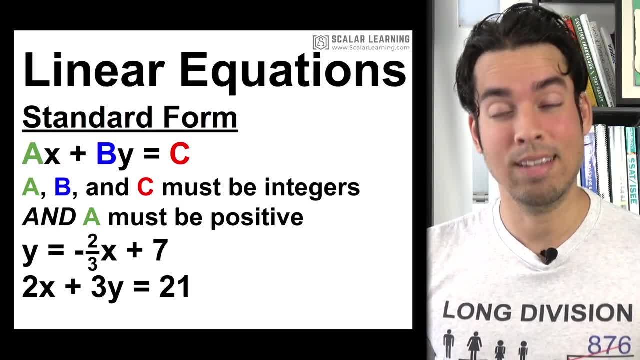 It just means that a must be a valid format of standard form. So, for example, if we look at, y equals negative 2 thirds x plus 7, that's in slope intercept form, The equation written in standard form would be: 2x plus 3y equals 21.. 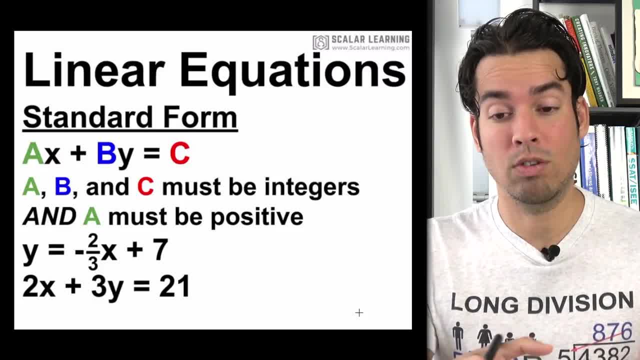 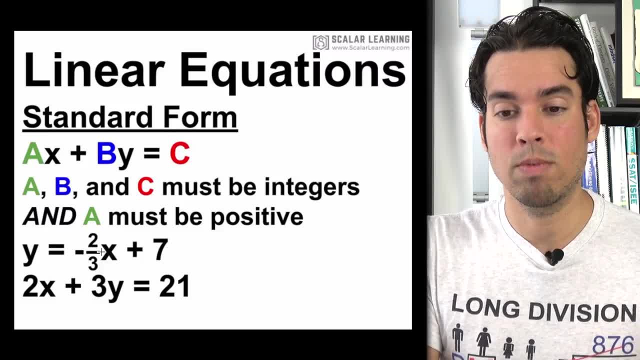 Now I'm going to show you how we go from that slope intercept form to standard form, how we get there, And essentially we want to think about isolating that constant. That's really what it's all about. So if I, for example, take this format, first thing I'm going to do is I'm going to add: 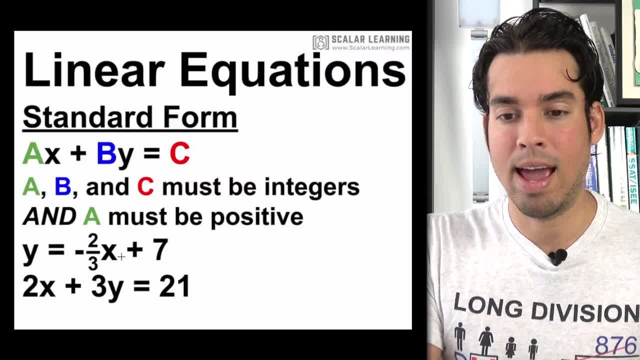 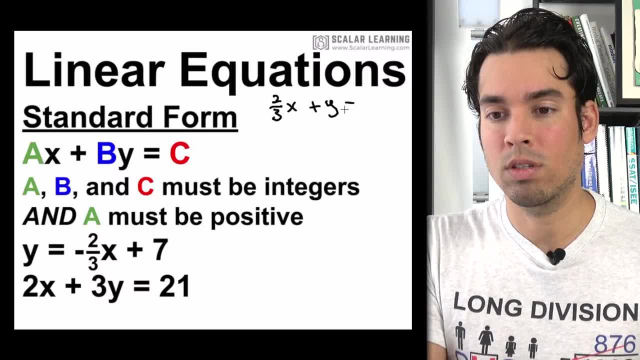 2 thirds x to the other side. So let's start up here. I'm going to add 2 thirds x to the right side and I get 2 thirds x plus y equals 7.. Okay, that's excellent, And then the last thing I need to do is: I can't have a fraction here, right? 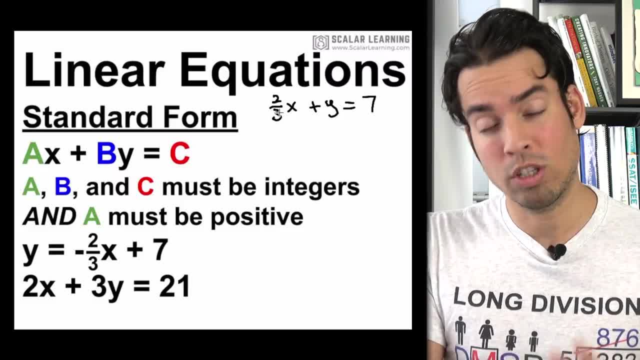 I need that 2 thirds out of there. So I'm not going to multiply by the reciprocal, which a lot of people think like, hey, I'll multiply by 3 halves. get rid of the fraction That's going to create fractions here and here. 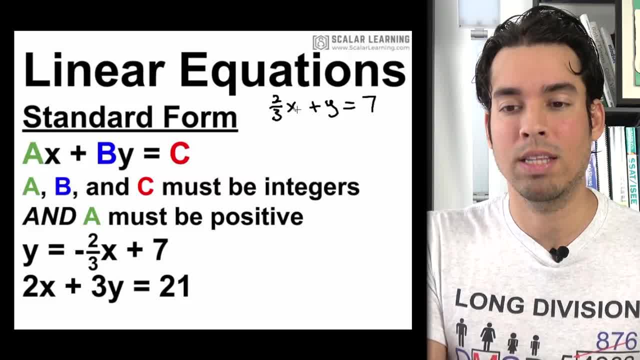 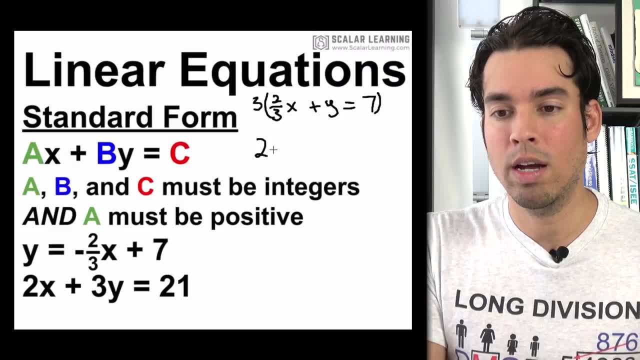 So instead, I'm going to look at that denominator and I'm going to multiply everything by that denominator, which is 3.. So I'm going to multiply this whole equation by 3.. 3 times 2 thirds is just 2x. 3 times y is 3y, and then 3 times 7 is, of course, 21.. 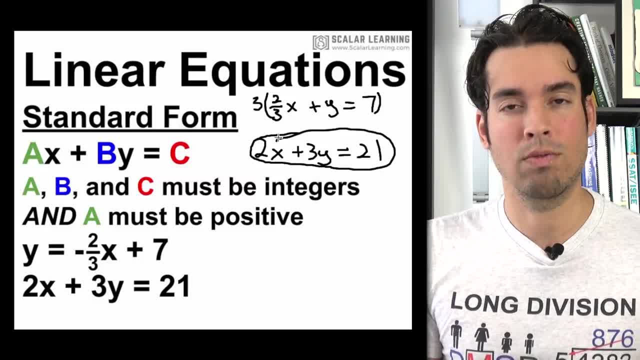 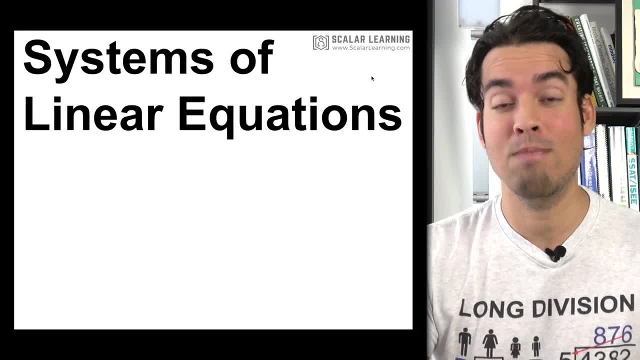 So that's how we go from slope intercept to standard form. Next we're going to talk about another huge topic involving linear equations, which is systems of linear equations, And that sounds really complicated, but really all it is is two lines could be more than. 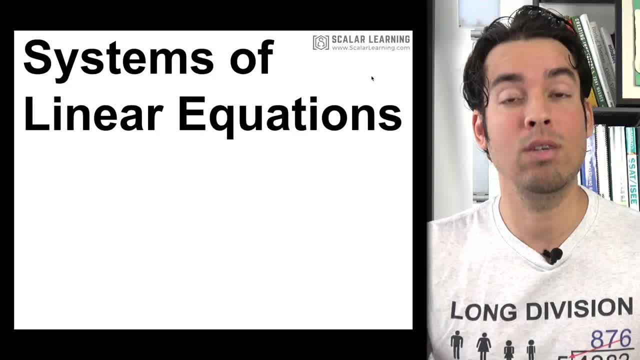 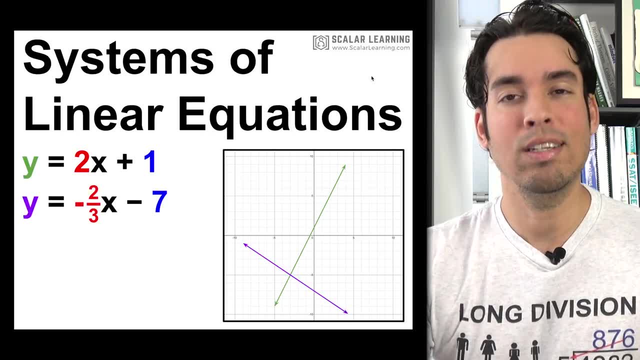 two, but usually on the SAT it's just two lines. It's two lines and we're seeing where they intersect. So again, if we take this example of y, y equals 2x plus 1, that's the green line, and y equals negative 2 thirds x minus 7,. 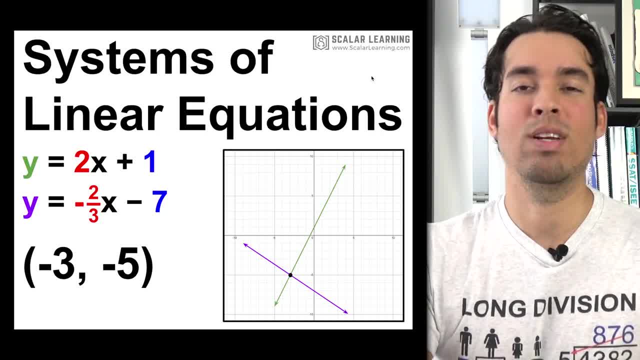 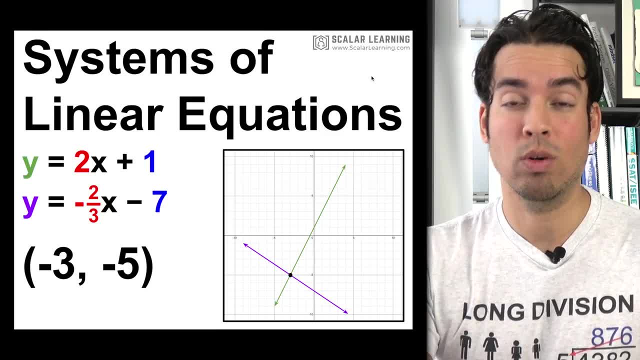 the solution to the system is that intersection point of negative 3, negative 5.. So that's it Again. it's just the intersection of the two lines and that particular coordinate where they intersect. Now, when we talk about systems of linear equations, what I previously showed you is: 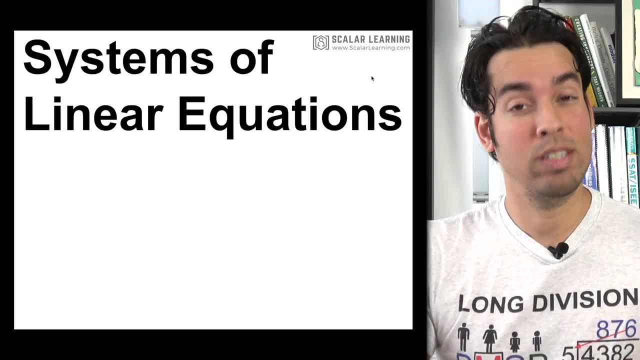 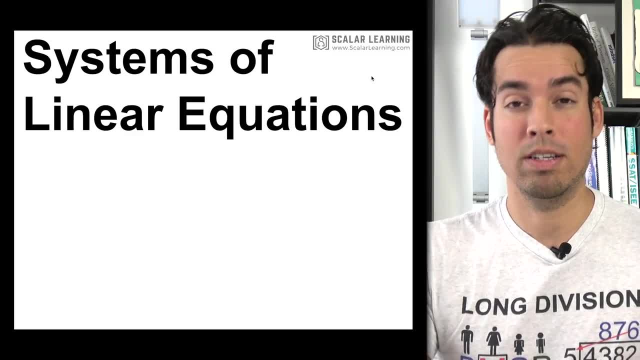 how to look and solve from a graph. But we may not always have a graph and we may not always want to make a graph because it takes a lot of time. So we're going to solve a system of linear equations algebraically. The first one is called substitution. 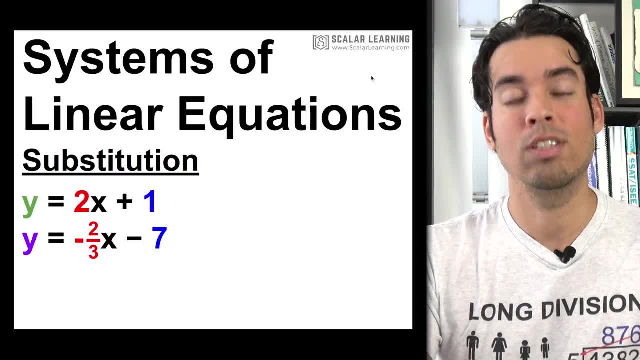 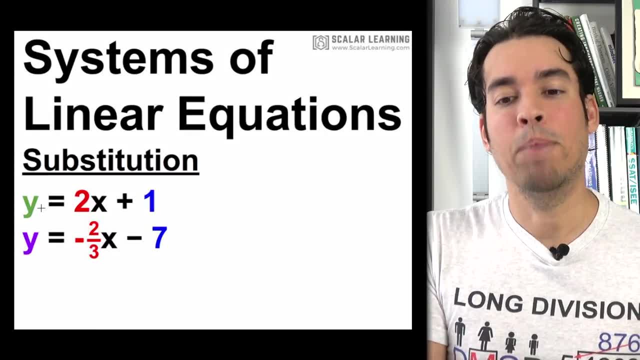 So, in substitution, what we're doing is, again, I'll take these two equations and we're going to substitute one into the other as long as y or x has already been isolated. In this case, both the y's are isolated in both the equations, so it makes it really 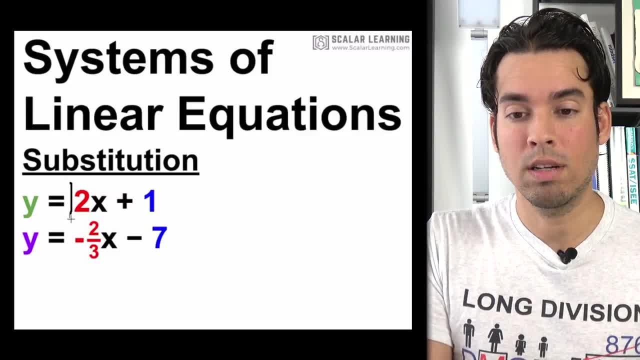 easy to sort of substitute, So I can say, like, well, wait a minute. since I'm looking for a point where these guys intersect and y already equals this, I'm going to plug this value in for the y down there They're x and y. 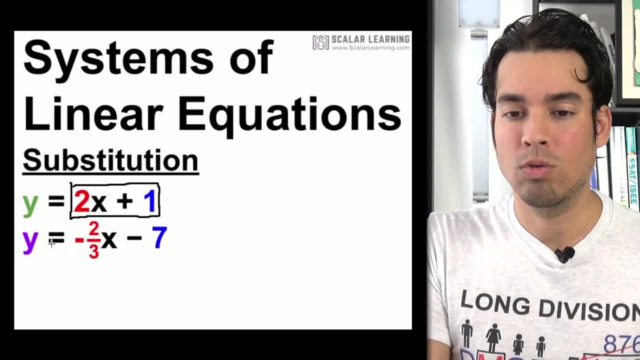 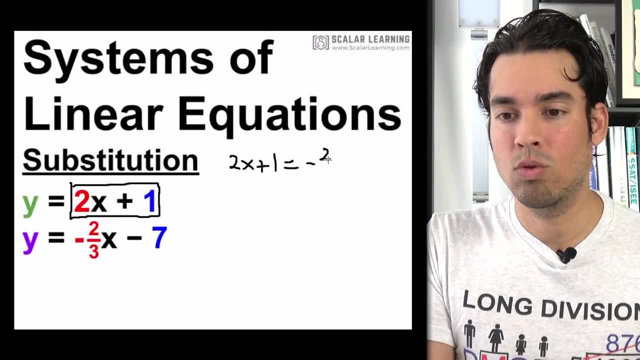 And y is our equivalent at this point of intersection, so I can do that. So instead of that y, I'm now going to write 2x plus 1, and this equals negative 2 thirds x minus 7.. And now all I've got to do is get the x's together. 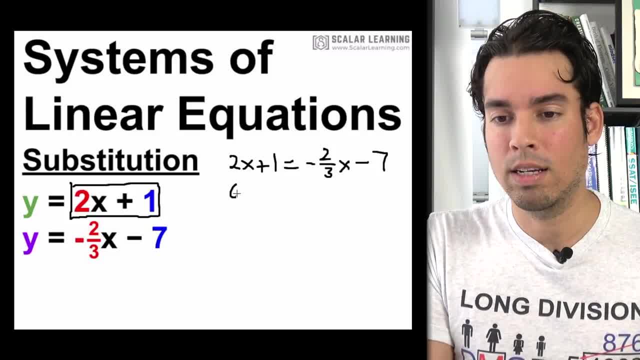 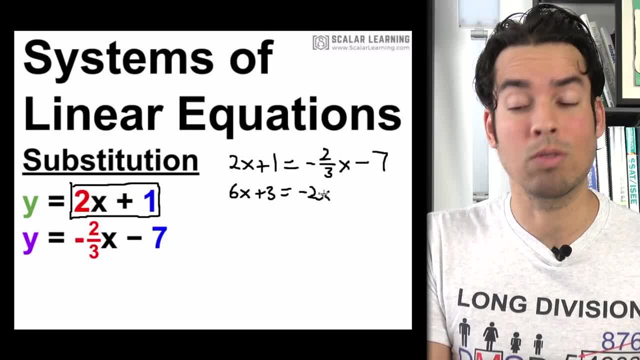 First, I don't want to deal with that fraction, so I'm going to multiply everything by 3, and I get 6x plus 3 equals negative 2x right Negative 2 thirds times 3 is negative 2x. 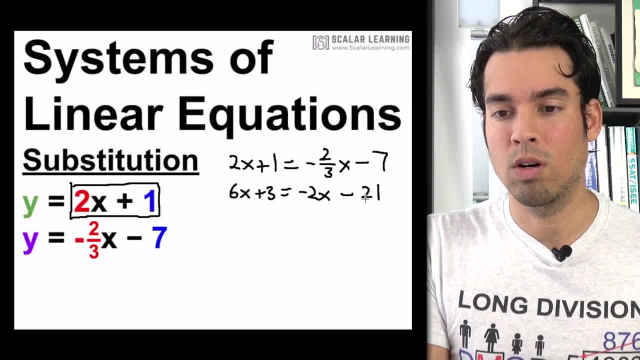 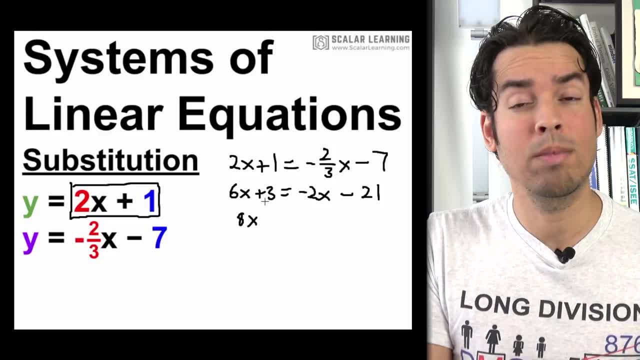 And then this times 3 is Minus 21.. So I will now add 2x to this side. 2x plus 6x is 8x, And then simultaneously I'm going to subtract 3 from both sides and negative 2, so that 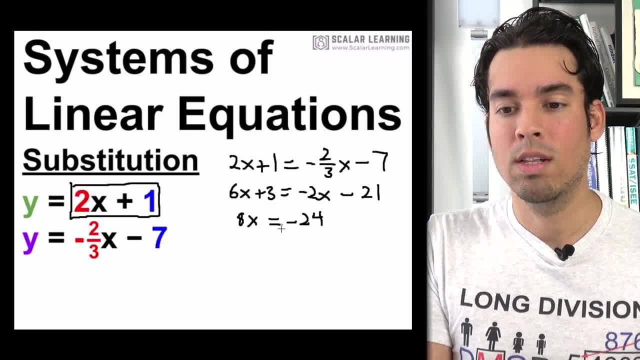 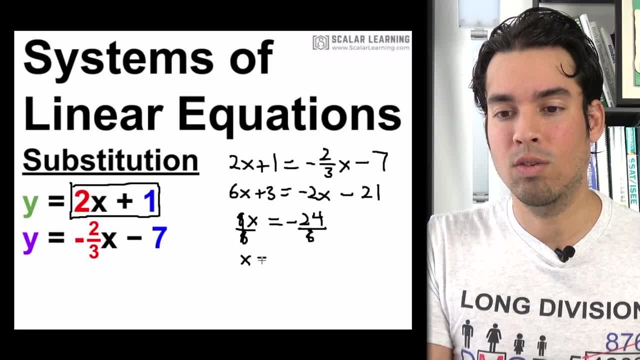 3 goes away. Negative 21 minus 3 is negative 24.. Last but not least, we're going to divide by 8.. And guess what? X equals negative 3.. And this is exactly what we got when we graphed it and we looked at the coordinate and the. 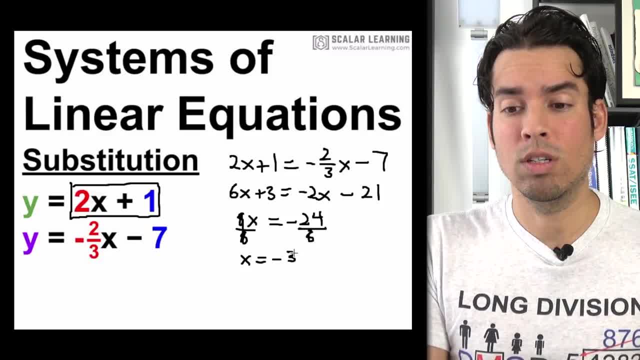 corresponding value on the graph was negative 5.. Now we're going to do this, but we're going to do it algebraically. So what do I do with that negative 3? I can now plug it into either equation and solve for y. 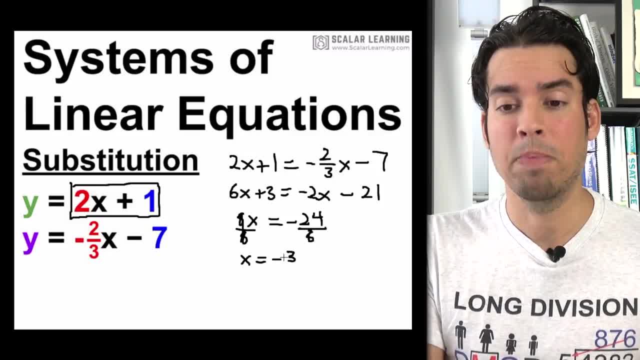 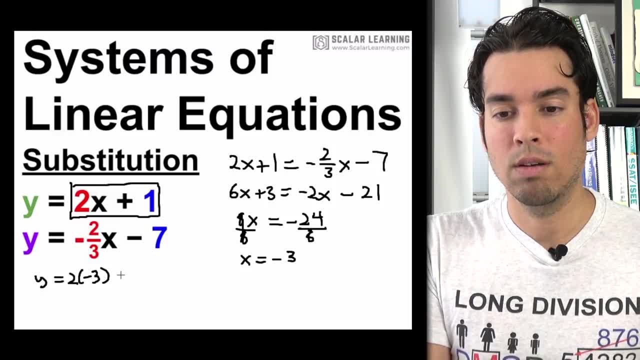 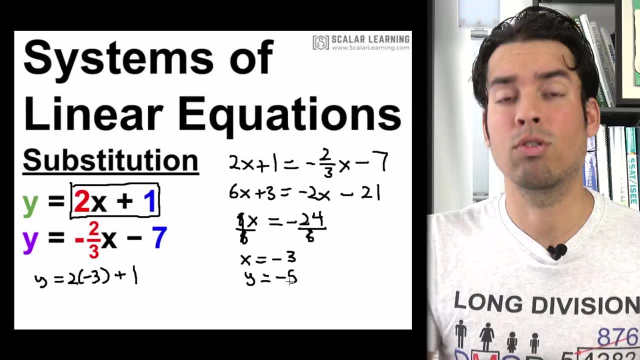 I should get the same value for both equations, if I've done this correctly. So if I plug in a negative 3 into this, I get y equals 2 times negative 3 plus 1.. That becomes negative 6 plus 1, and therefore y equals negative 5.. 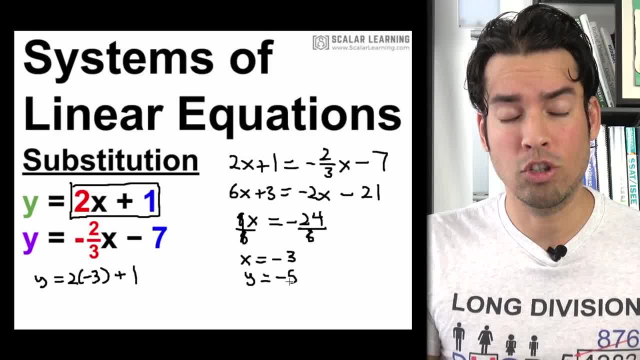 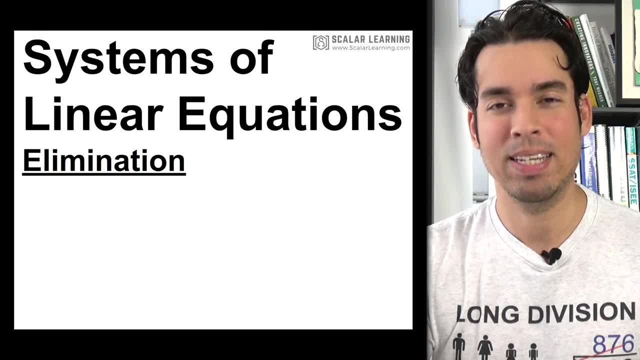 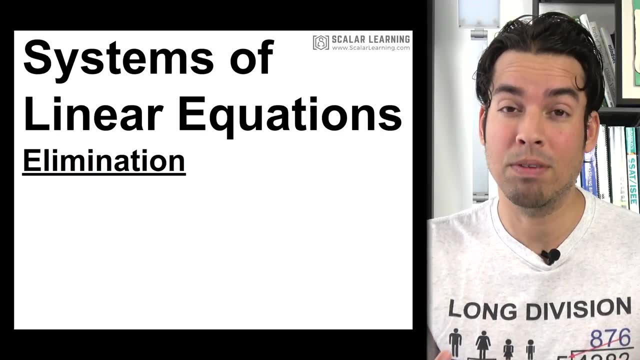 So there we have an algebraically derived equation. Next we're going to talk about solving systems of linear equations using the method of elimination. So elimination is actually my favorite. Whenever I can do it, I do this instead of substitution. I find it to be easier and a slight bit faster. 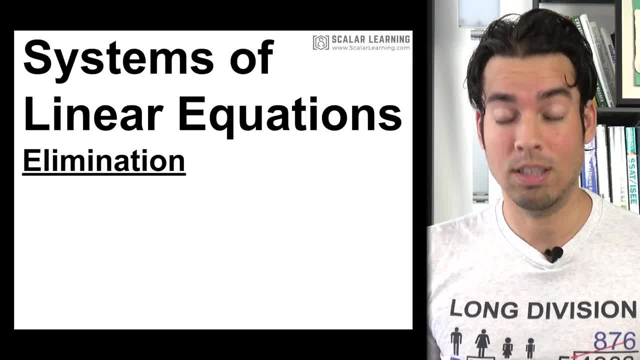 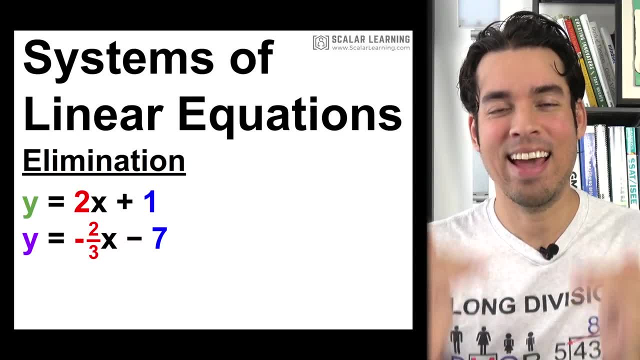 However, there are certain situations where substitution is just the better option. But what is elimination? Elimination is where we take two equations and we kind of match them up and then add them together, Whereby we're adding them in a way Where one of the variables cancels out. 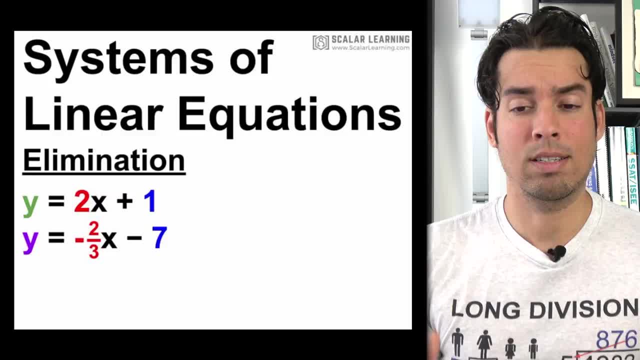 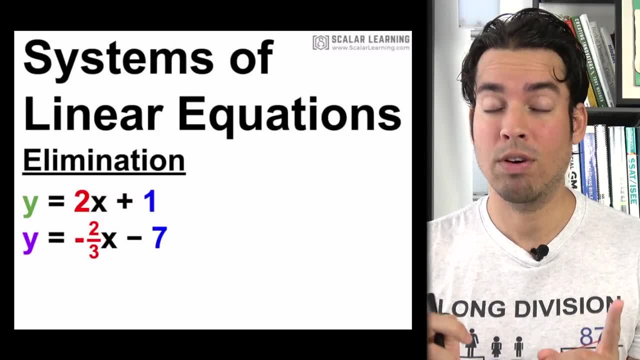 Okay, so I'm going to show you how to do this now. So again, I've chosen the same equations and you'll notice that the y's are perfectly matched up and they both have a coefficient of 1, and that's very important. 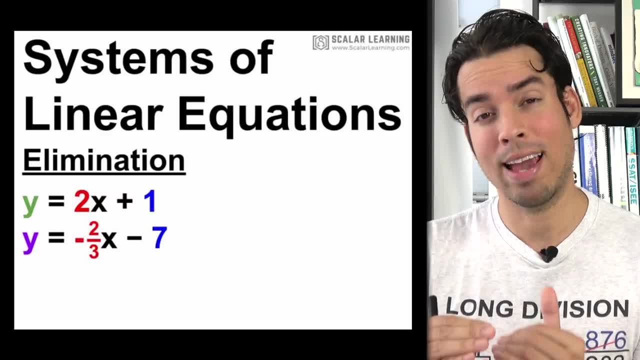 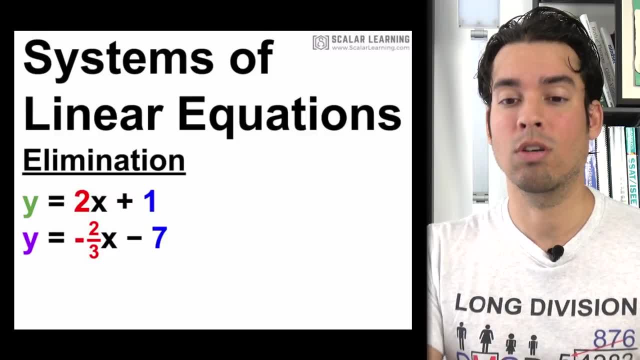 But I'm going to show you a different way to do this, because I want to focus more on the x's and show you the process of how we have to match up coefficients to properly eliminate in any situation. So I look at this and I've got a 2x here, right? 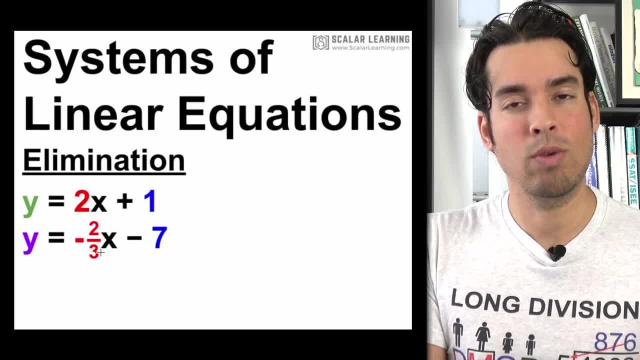 Theoretically. I'd love to be able to have a new equation, So I'm going to do this. I'm going to get a negative 2x on the bottom, and I'm going to show you why. So, first of all, how do I get a negative 2x on the bottom? 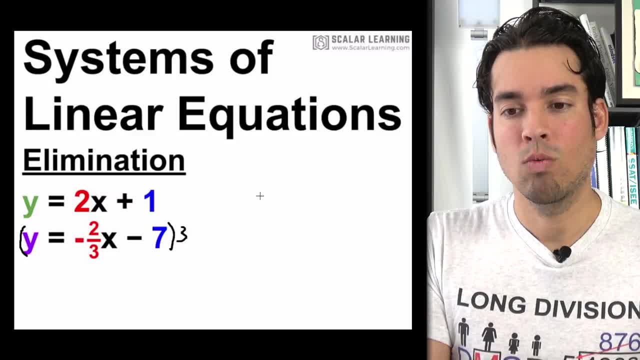 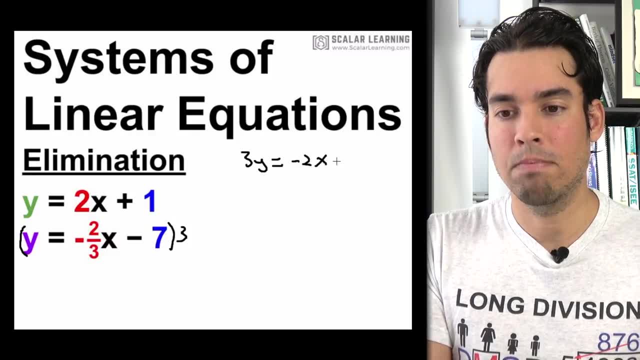 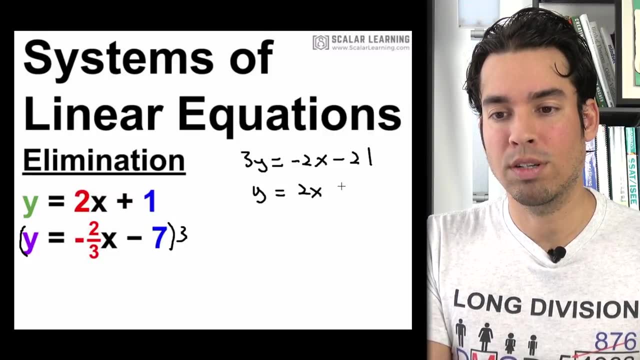 If I multiply this entire equation by 3, watch what happens. I get 3y equals 3 times that is negative 2x and then minus 21.. Now I'm going to take my original, my top equation, which is: y equals 2x plus 1 and. 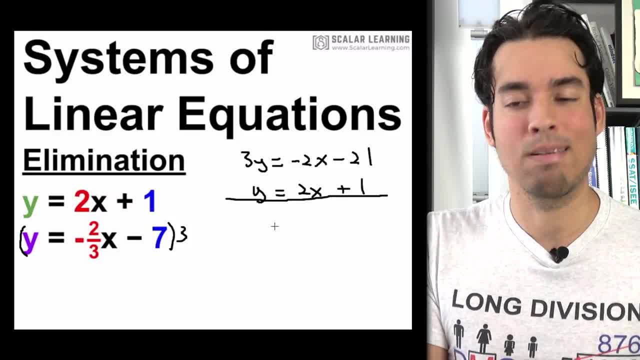 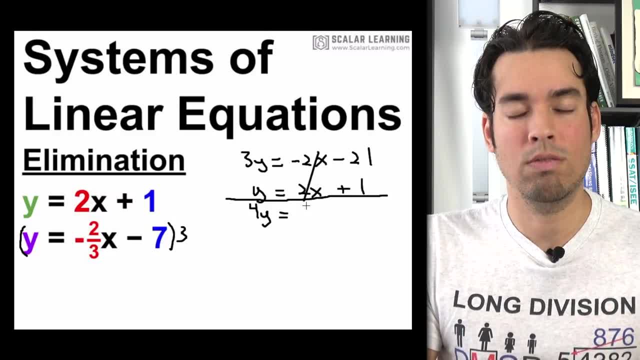 I've got something really special. Now I can add these together. I can combine them. I can say 3y plus y is 4y, 3y equals that's zero. So now I've canceled out one of the variables. 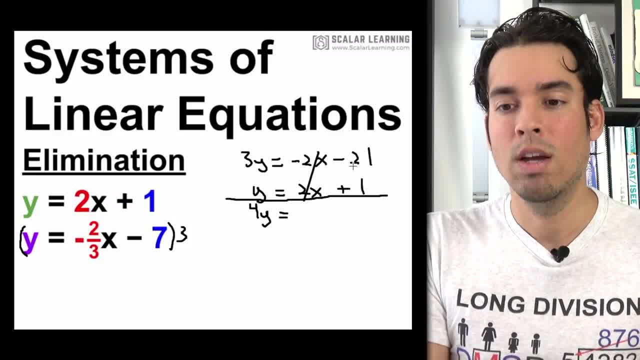 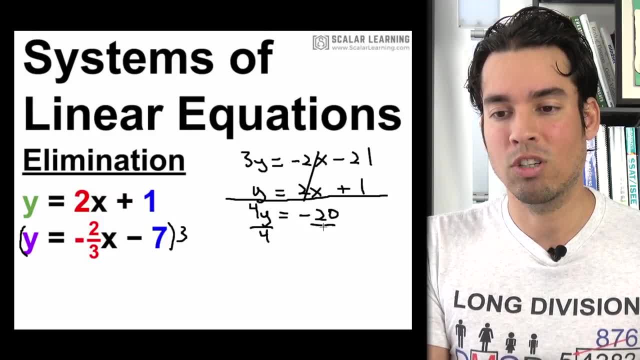 I've got a single equation with a single variable. Now I can solve. And then I got negative 21 plus 1 is negative 20, all right, Now how do I isolate? Simply divide by 4, inverse operation of multiplication, and I've got y equals negative 5.. 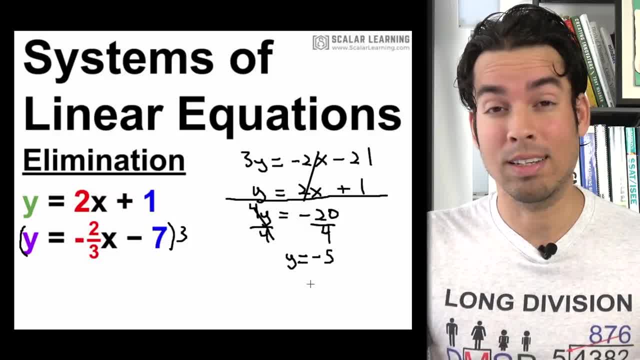 Terrific- And once again this matches up with our previous answer- that we got in substitution To get the x value. I just take this negative 5 and plug it into either equation. I'm going to plug it into the top one. 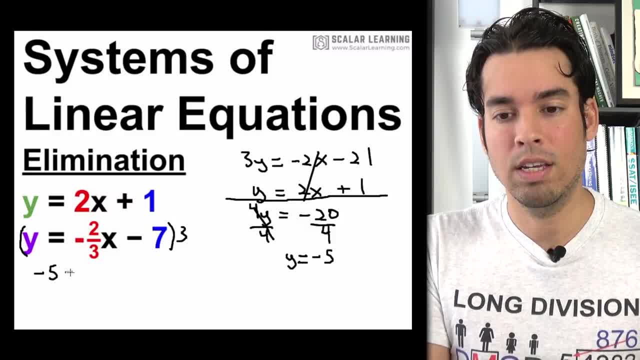 That feels easier to me. So then I got negative 5 equals 2x plus 1.. By subtraction we're going to isolate, I'm going to subtract 1 from both sides. Boom, I got now negative 6 equals 2x. 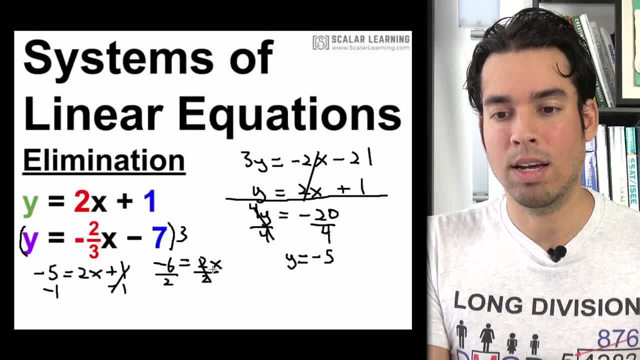 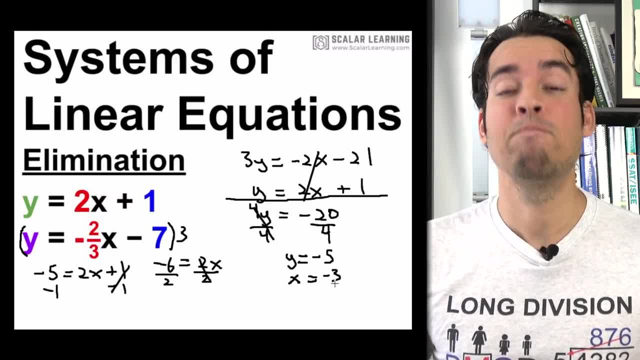 And last but not least, divide by 2.. Divide by 2. And I've got x equals negative 3.. So again you can see. whether we graph, whether we substitute, whether we eliminate, we get the same answer every time, which is a coordinate pair of negative 3 times 2x. 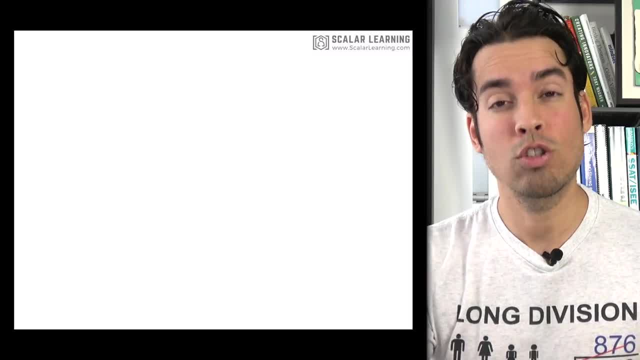 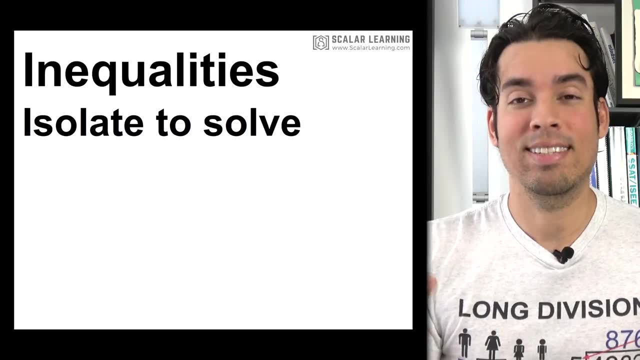 All right, So that's negative 3 comma, negative 5.. Next we're going to talk about inequalities. Now, inequalities are another thing that the SAT loves to test on, the College Board loves to test, And the same key exists. we're going to isolate to solve. 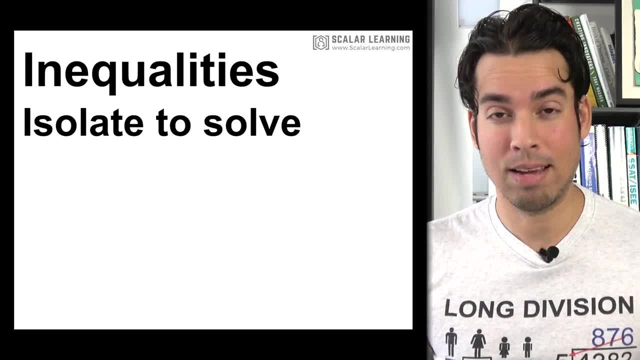 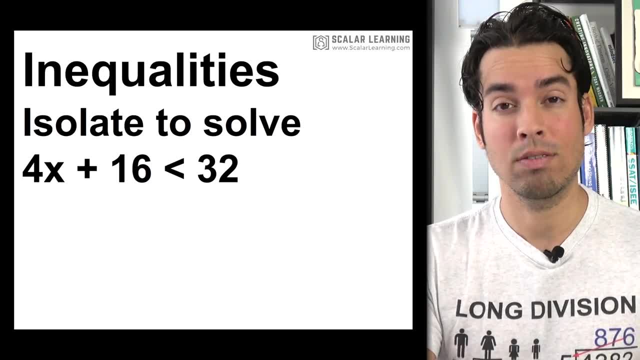 So nothing changes here in terms of how we're applying our same methodologies. If we take this example of 4x plus 16, is less than 32, once again, I want to get my variable by itself. So, as we get the variable by itself, what we're going to do is again move the thing. 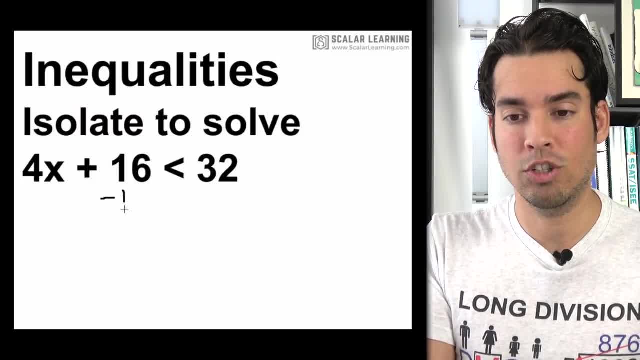 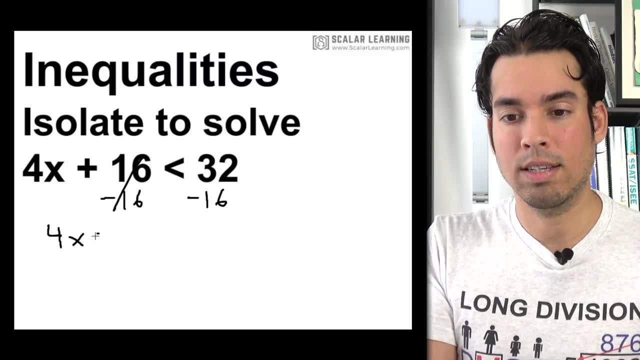 farthest away from the variable first, which is that 16.. And the opposite of addition, It's subtraction. So we're going to subtract both sides by 16.. Now I have: 4x is less than 32 minus 16, which is 16.. 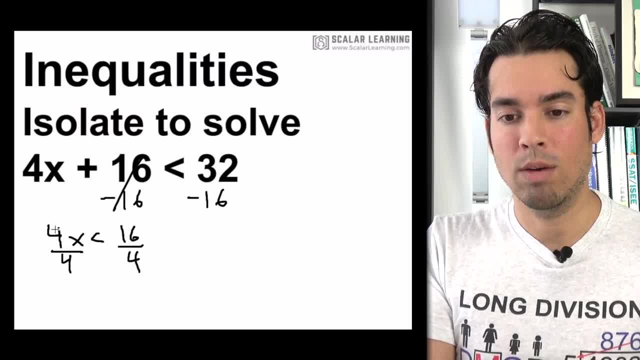 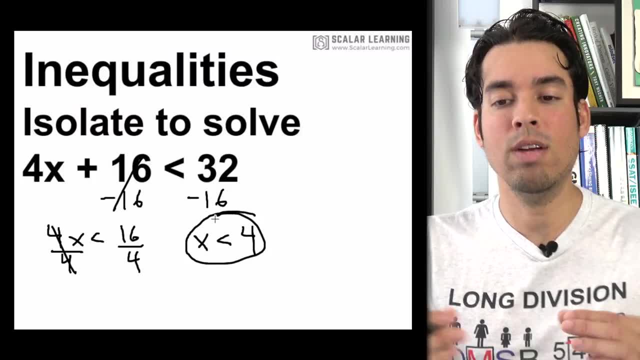 Last but not least, divide by 4.. Get rid of that 4. And we've got. x is less than what's 16 divided by 4? That is 4.. So once again, we've used variable isolation. We don't have a specific one solution. 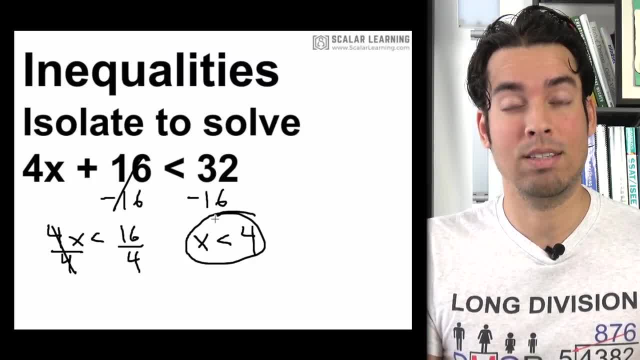 This is actually an infinite amount of solutions, right? because it's everything that is less than 4. satisfies this equation? Meaning 3x is less than 4.. Satisfies this equation 3,, 2, 1, negative 100, negative a million, and so on and so forth. 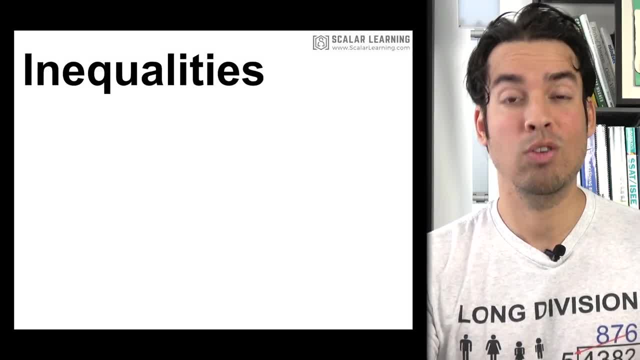 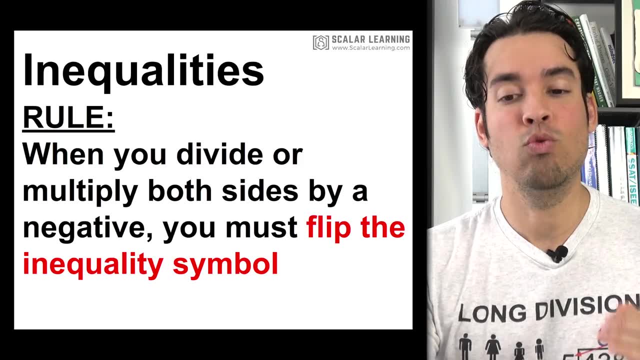 When we're dealing with inequalities, there is one rule that you've got to know, that is tested pretty frequently on this SAT, which is that when you divide or multiply both sides by a negative, you must flip the inequality symbol. So here's a quick example of when you must flip the inequality symbol to get the right. 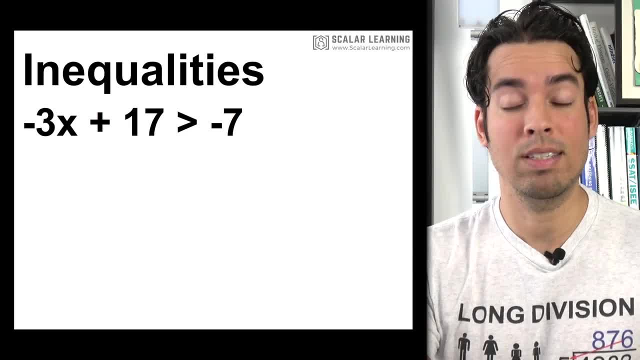 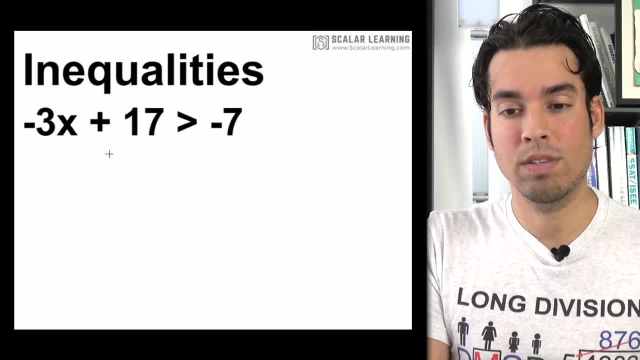 answer. So we've got this: inequality negative 3x plus 17 is greater than negative 7.. All right, Let's solve, Let's follow the standard protocol, Isolate. So first I'm going to get rid of the 17, because that's farthest away. 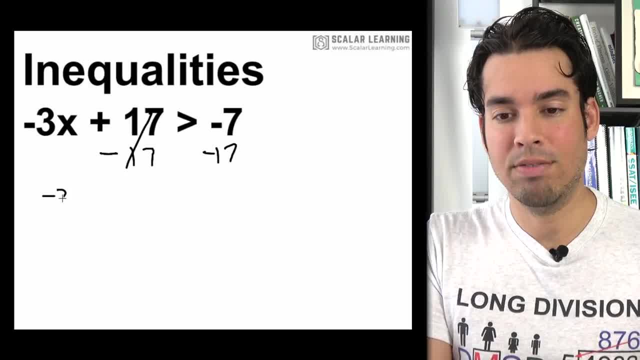 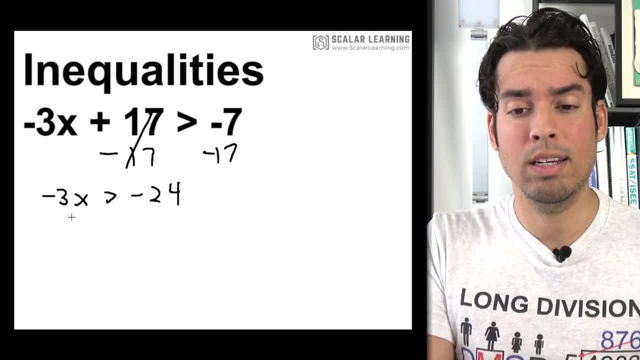 Let's subtract 17 from both sides and I get negative 3x is greater than negative 24.. Terrific. Now I have to continue to isolate. I need to get rid of that negative 3.. It's multiplying, So I'm going to divide. 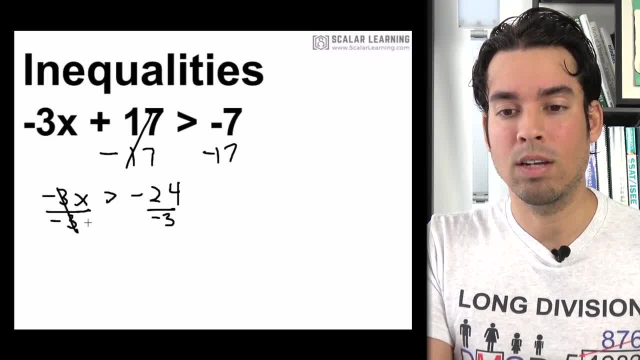 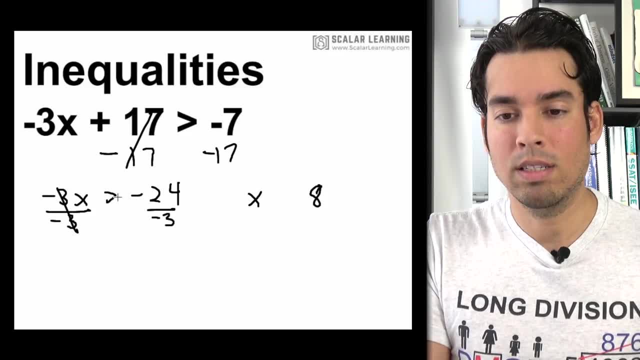 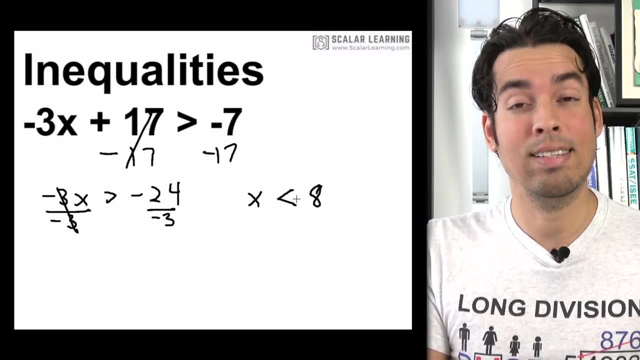 I'm going to divide both sides by negative 3 and we get: x is now here. negative 24 divided by negative 3 is 8.. But wait a minute. Normally I'd say x is greater than 8.. But because we divided by negative, we have to flip the inequality and I say x is less. 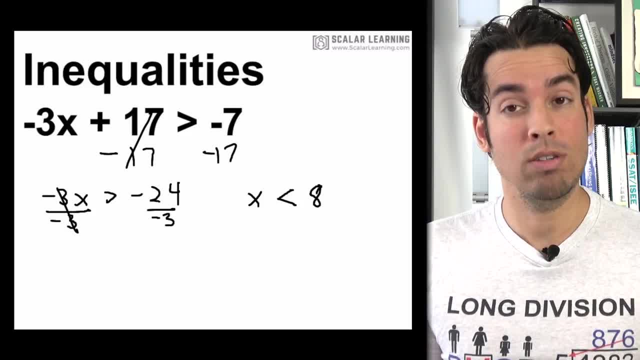 than 8.. Now, that might seem a little weird, but then you can try values out and plug them back in and you'll see that it actually works. So, for example, if I plug in a 7 here, I should get a true statement. 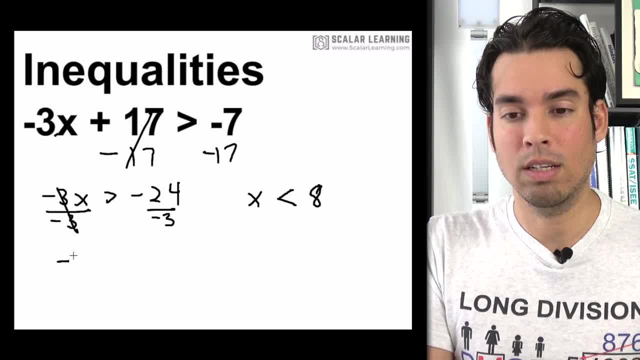 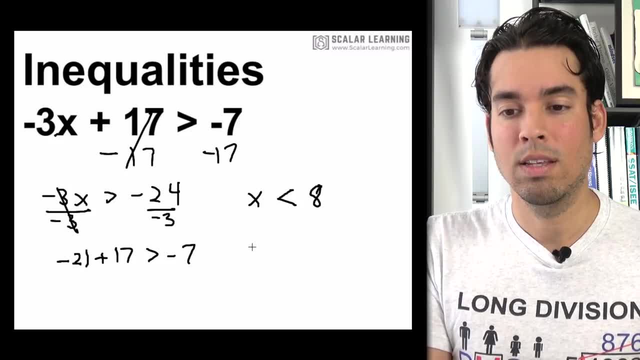 So if I plug in a 7, that'd be negative 3 times 7,, which is negative. 21 plus 17 is greater than negative 7.. What's negative? 21 plus 17?? That is negative 4.. That is negative 4.. 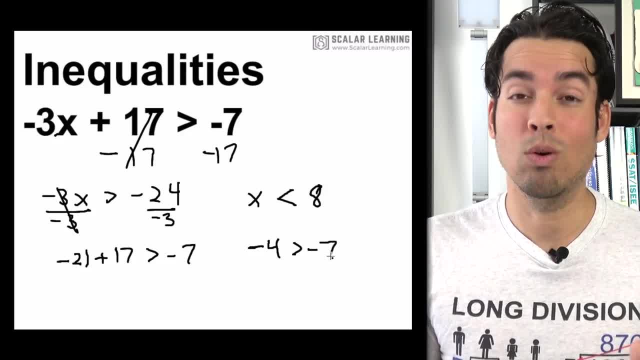 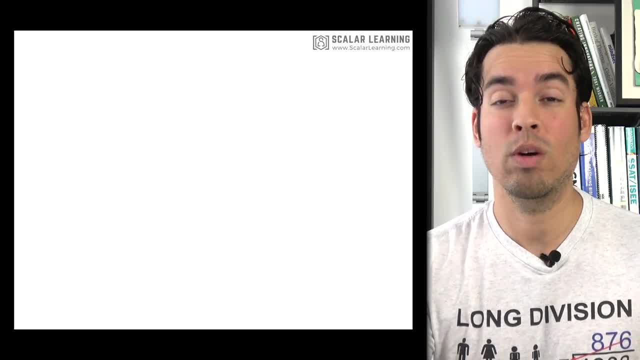 That is greater than negative 7.. Guess what? That's a true statement. Therefore, we know we've done this correctly. Now let's talk about how to graph these linear inequalities. Okay, Again, linear inequalities is just like a linear equation with y and x, but we have 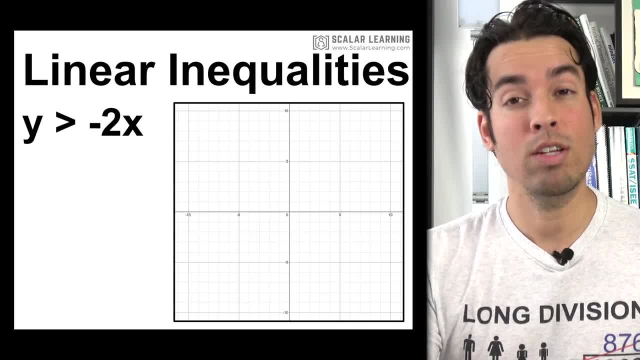 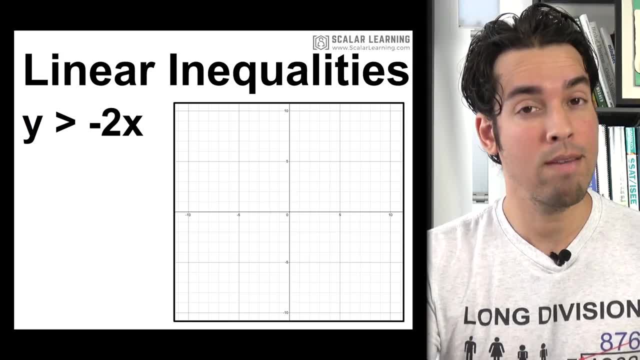 an inequality symbol instead. So, for example, if I have y is greater than negative 2x, the first step is we graph this just like: the line of y equals negative 2x. However, because it's a greater symbol, not a greater than, or equal to, not a less than, 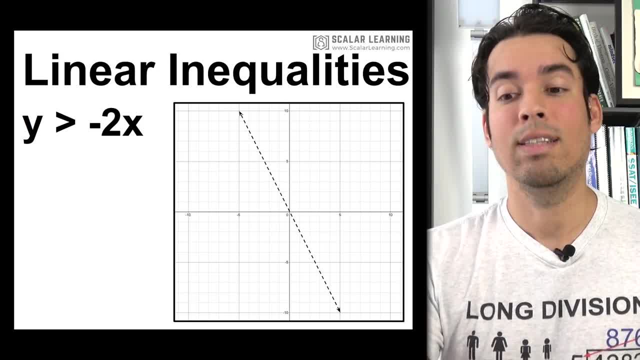 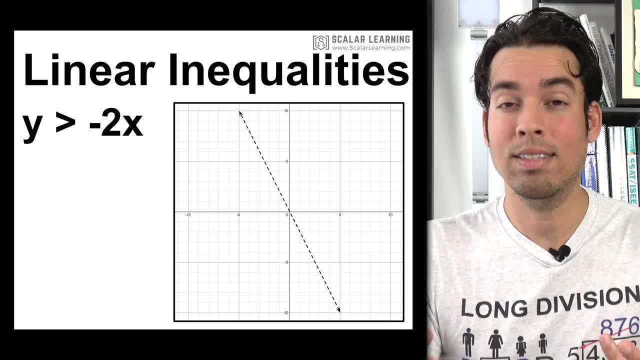 or equal to, we have to start with a dotted line. So that is literally the line of y equals negative 2x, except for it's dotted because we're representing that it's greater than meaning. the line itself is not an inclusive. 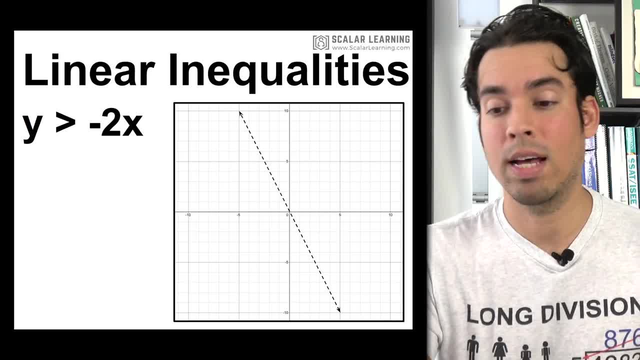 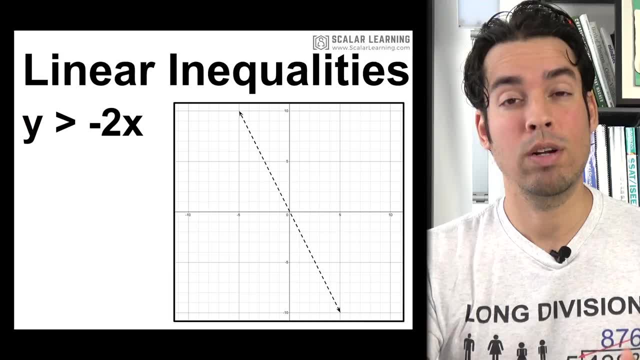 solution, but certain values bounded by that line are the correct values, are the solutions. So when we say, now we're going to graph y is greater than negative 2x, we need to shade because we need to cover that massive solution set of everything above this line of negative. 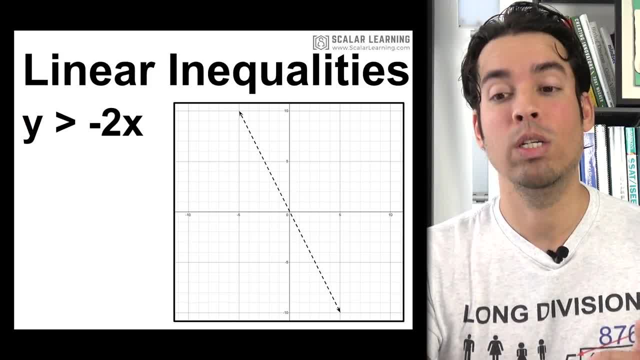 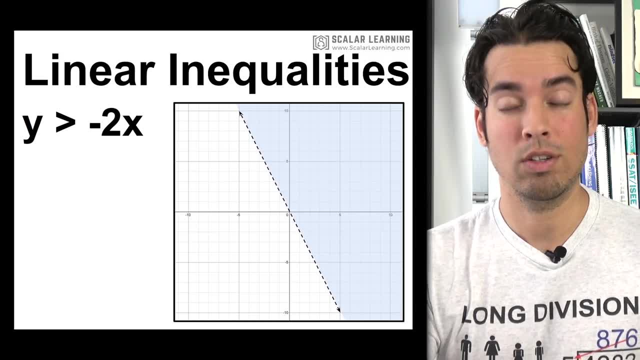 2x. So when we see that greater symbol, we know we have to shade that line. Okay, We have to shade above. So you see how that shading is going up from the line. That's how you shade a linear inequality, correctly. 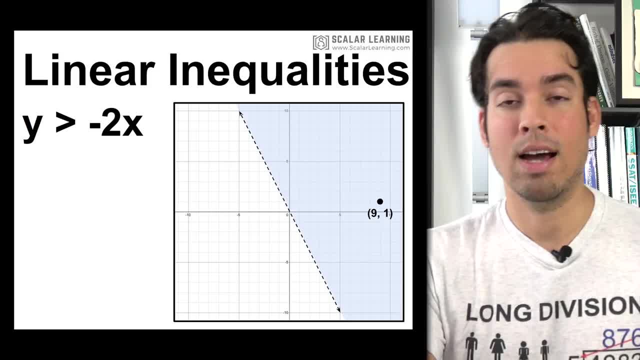 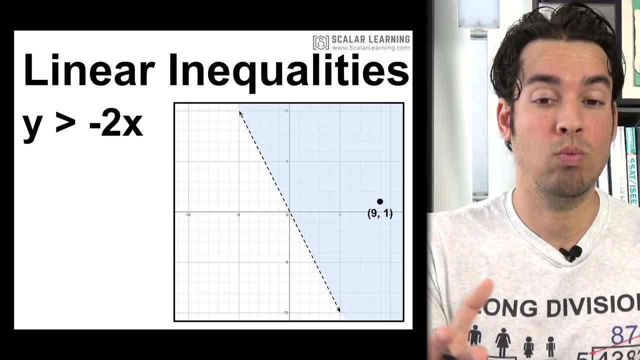 Now, when we think about solutions to this linear inequality, we can see that nine comma one is a solution. It's in that solution set. This is one of infinite solutions. and it works again because, again, if I plug in one for y and nine for x, I get one is greater than negative 18.. 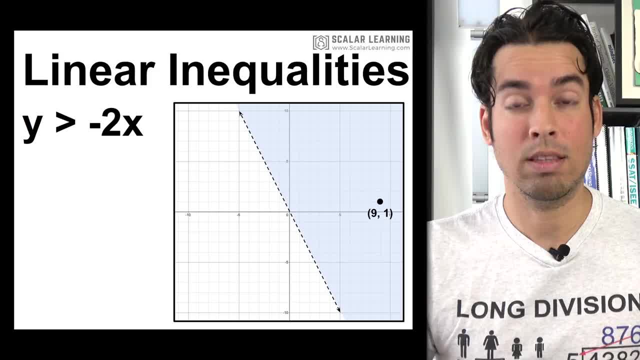 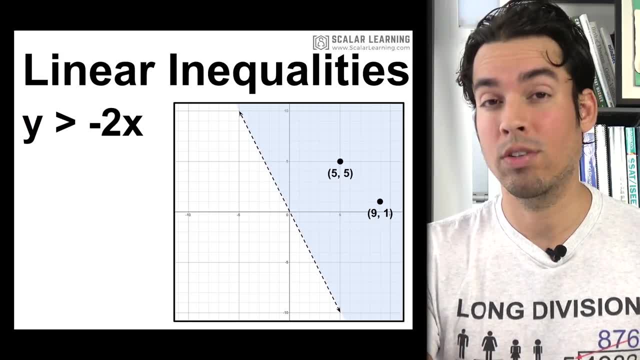 That's a true statement. that just helps us verify or validate the fact that we've graphed this correctly. Here's another solution of five comma five, and once again, if I plug that in, I get five is greater than negative 10, which is again a true statement. 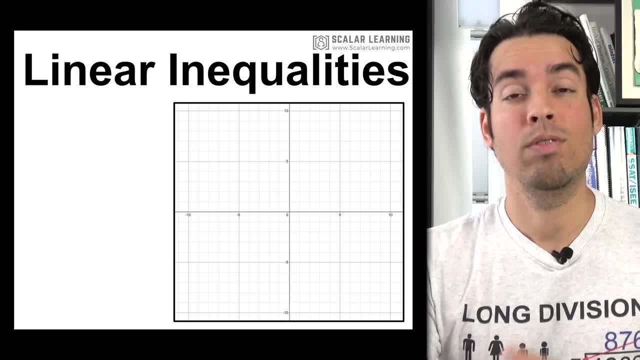 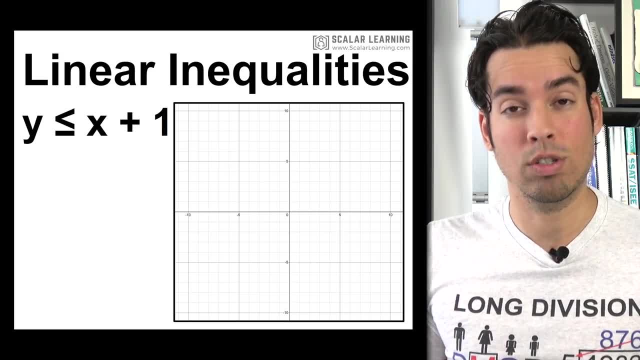 Now let's look at an equation where it's not greater than or less than. we've got an equal in there. So this is: y is less than or equal to x plus one. Now the line itself is also a solution, plus all the values less than that line, because 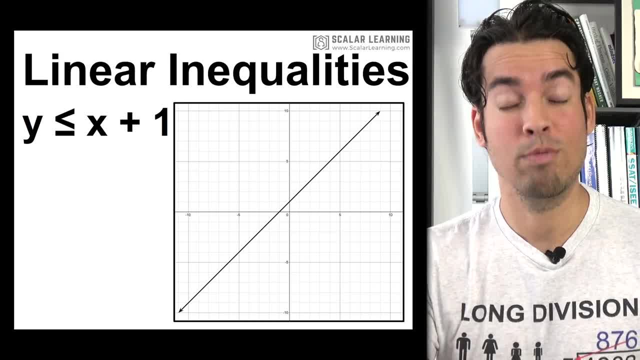 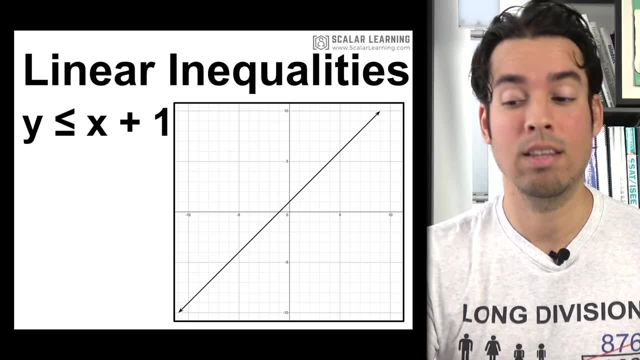 again, it's less than or equal to. So now again, we graph a solid line here, because it's less than or equal to, and that is the line of y equals x plus one. Now, where do we shade? Well, it's less than. therefore, we shade below right. 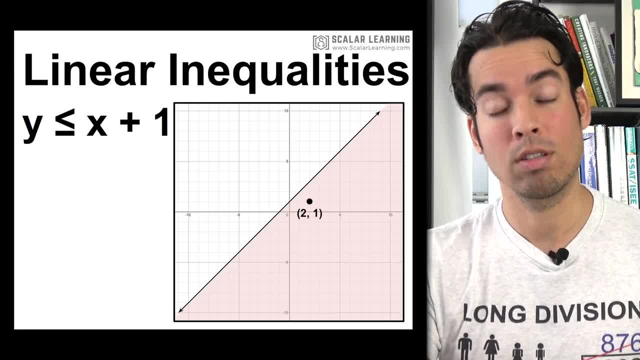 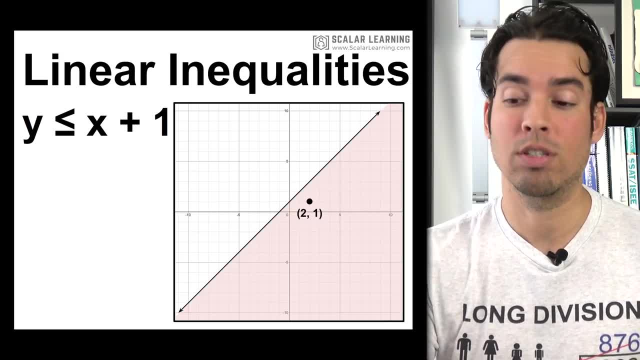 So it's below, And here we see two comma one. That's in the solution set. That makes sense. If I plug in two for x and one for y, I get one is less than or equal to three, which is a valid statement. 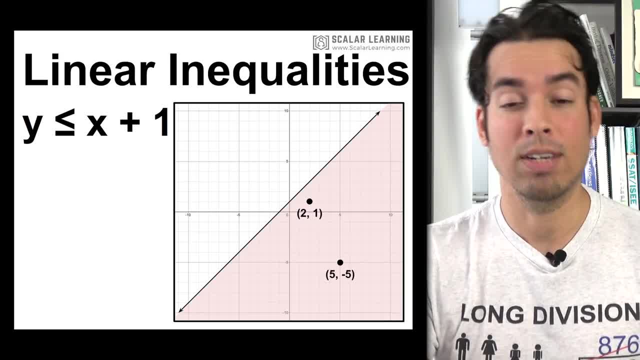 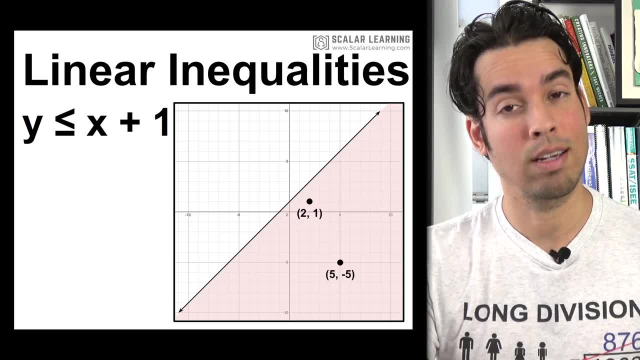 Here's another coordinate in the solution set, which is five comma, negative five Again. if I plug in negative five for y and five for x, I get negative five is less than or equal to six- Again a valid statement. Now let's talk about systems of linear inequalities. 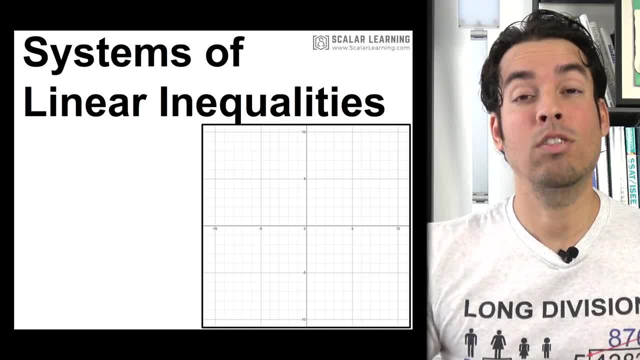 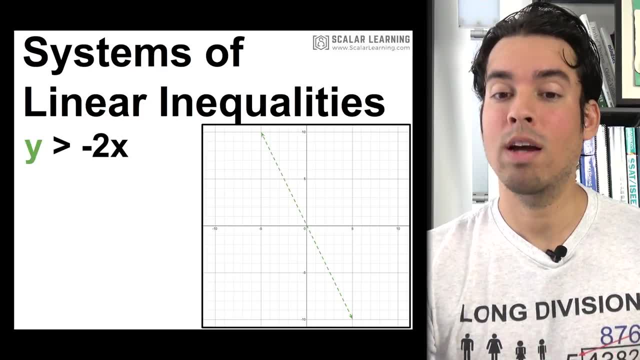 Just like systems of linear equations is two or more lines, systems of linear inequalities consist of two or more linear inequalities. So again, let's go back to our initial two examples. We've got: y is greater than negative two x, where we're again shading above that line. 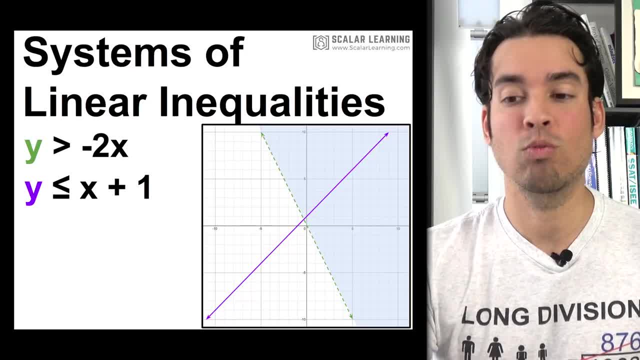 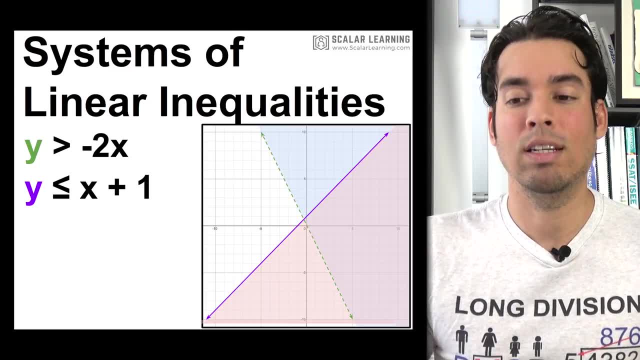 Then we've got: y is less than or equal to x plus one and we're shading below. Now, when we have a system, we are looking for the overlap of the shading and you can see to the far right that dark purple section Where it's both. we've got the red and the blue shading. 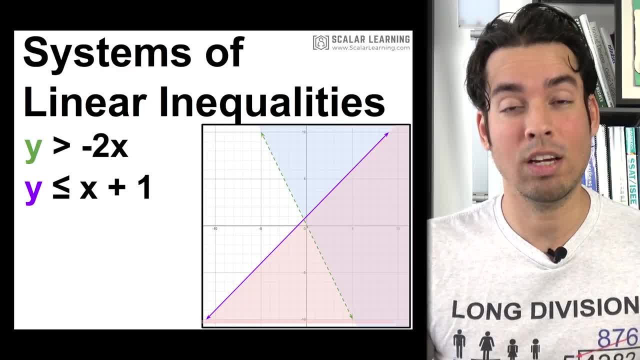 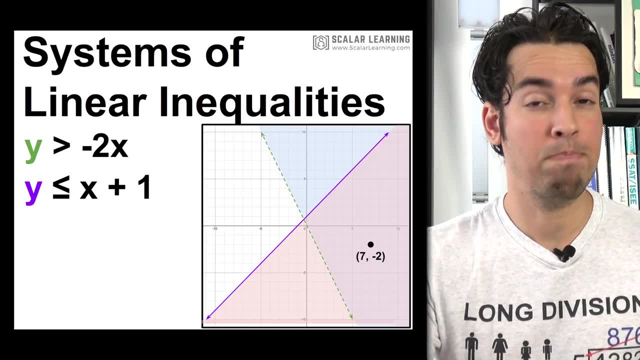 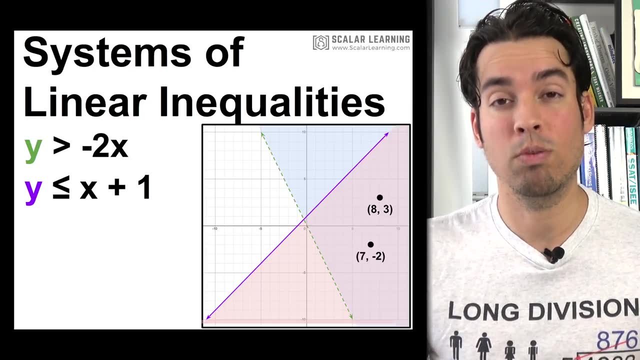 That is our limited solution set. So we're looking for the intersection of those two zones. In this case we see that seven negative two will be a true solution for both of these linear inequalities, just like eight comma three. So if we were to plug these in to both of these linear inequalities, they would both 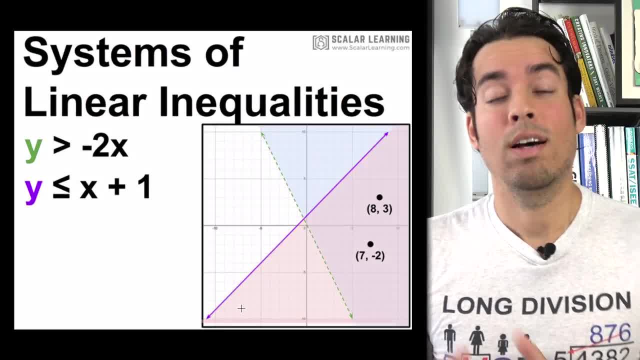 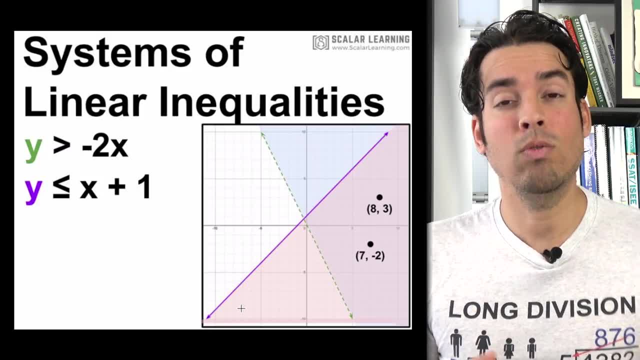 be valid statements. Now just a quick note. If you're asked to assess a system of linear inequalities and determine whether or not a particular coordinate Satisfies, Assess the system. I don't necessarily recommend trying to merge the inequalities like we do with substitution.